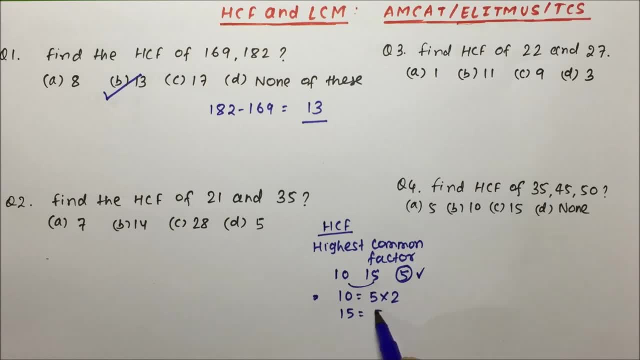 then you will write 5 into 2.. 15, if you will factorize, then you will write 5 into 3.. Now, highest common factor. That means in the factors we have to select the highest common factor. So you can see, 5 is the 5 is the highest number, which is common in both 10 and 15 factor. 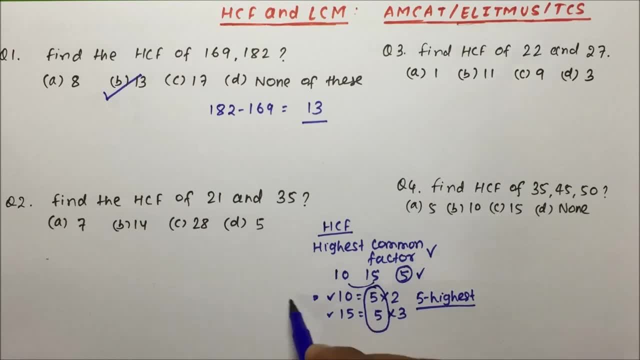 So SCF of this number will be 5, right. And what is the trick here? 10 and 15 calculate the SCF. Sorry, find out the difference. If you find out the difference, difference will be 5.. That means SCF of this number is 5, right. Now let us see. 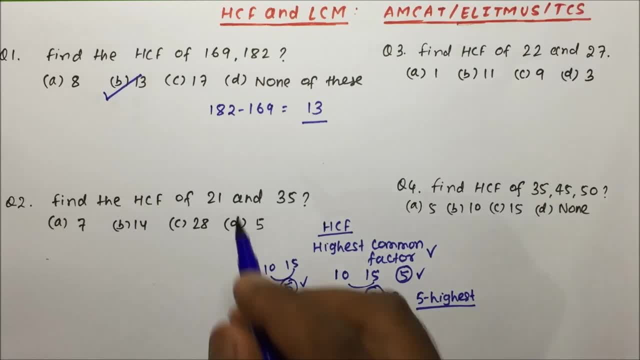 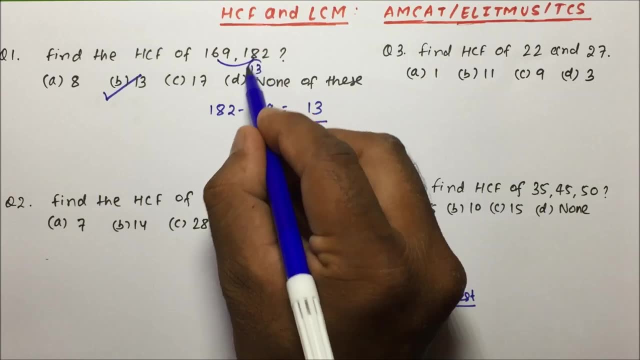 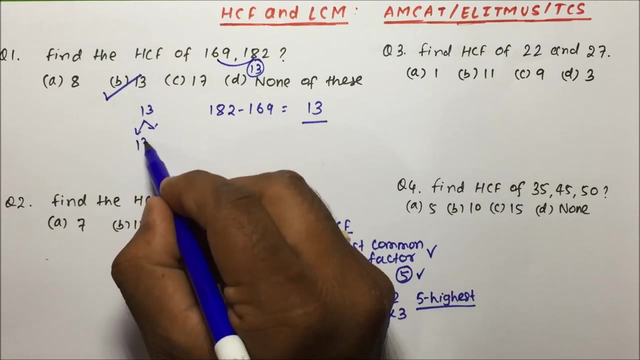 the other problems, then your concept will get clear, right, Okay. So question number 1, what I did? I calculate the SCF of 169 and 182. So take the difference. So difference is 13 here. So either 13 or either 13 or the factor of 13.. So the factor of 13 will be what? 13 and 1.. Because 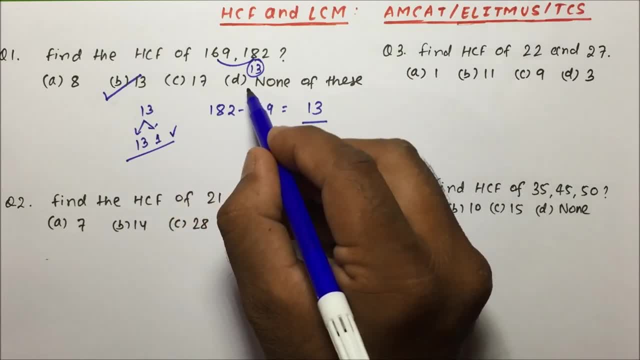 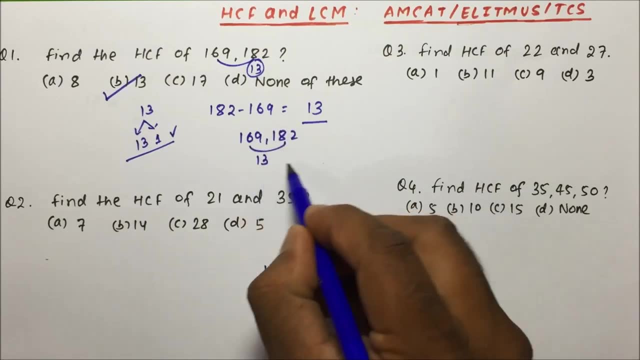 13 is a prime number, will be, will be what Will be your SCF, right, Okay. So when you take the difference, friends you see here, So when you take the difference, difference is 13,. right, Okay, And 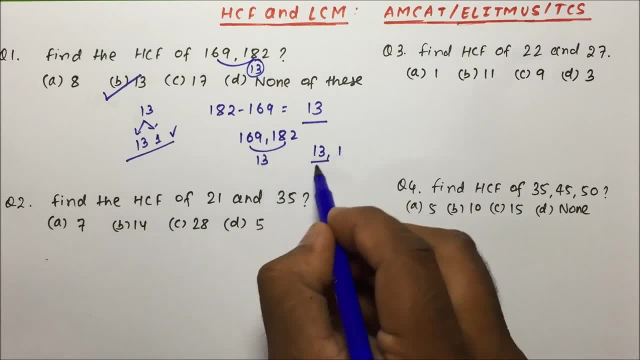 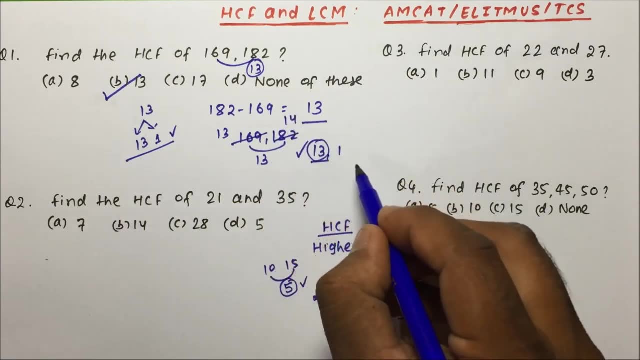 13 is having only one factor: 1.. So first divide this numbers by 13.. So 13 will divide this by 13 times and 13 will divide this by 14 times. That means my SCF is 13.. If it will not get divided, 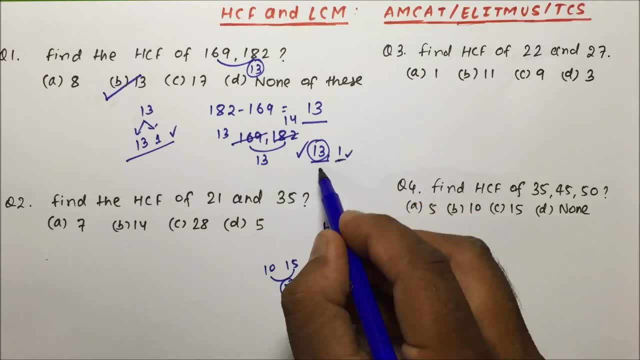 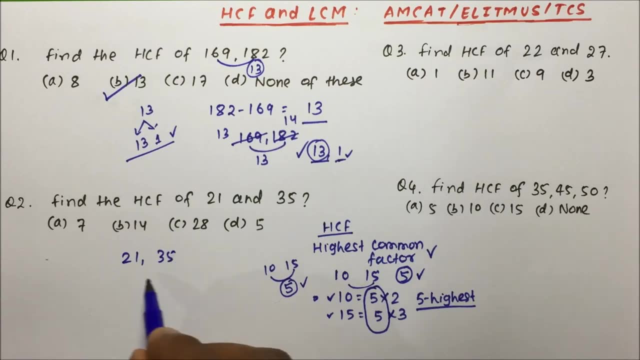 by 13,, then 1 will be the SCF, right, Okay? But here we are able to see it is getting divided by 13. So SCF is 13.. Now find the SCF of 21, comma 35. Now, what will be the difference of this number? 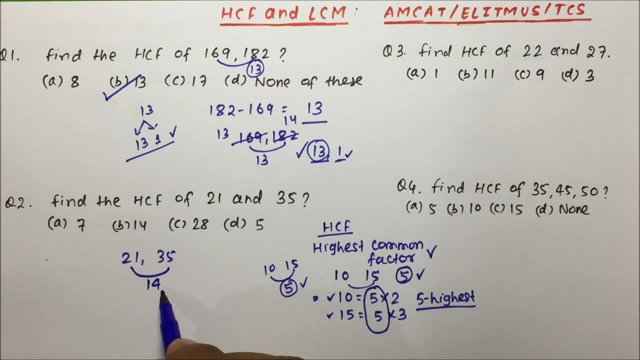 So difference of this number will be 4 and 1, 14.. So 14 should be the SCF, right, 14 should be the SCF. But you see is 14 is able to divide both the numbers. No 14. 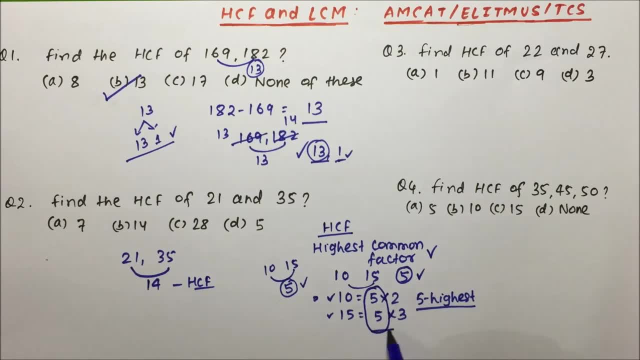 is not able to divide any of the numbers, right? See SCF means what. Here you can see: 5 is the SCF, So 5 is the SCF means 5 should be able to divide 10 and 5 should be able to divide 15.. 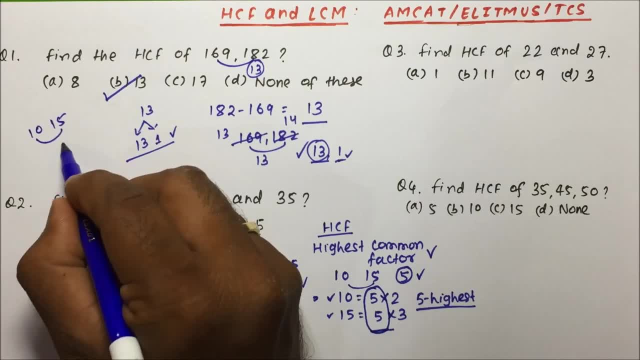 See, as I told friends, 10 and 15 will be the SCF. So take the difference. Difference is 5.. Now, is 5 is able to divide both? Yes, 5 is able to divide both. That means 5 is the. 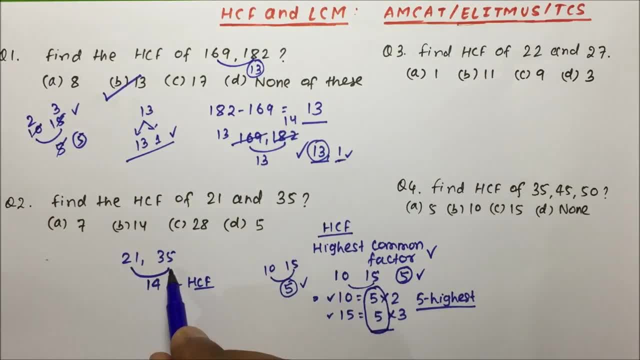 SCF, right Okay. But here you see, 14 is not able to divide 21,, 21 and 35, right okay? Then what we will do? we will calculate the factor of 14.. 14, if we will divide by 2, then 7 times. Now you try to divide this by 7 times, So 7 will divide this by 3 times 7 will. 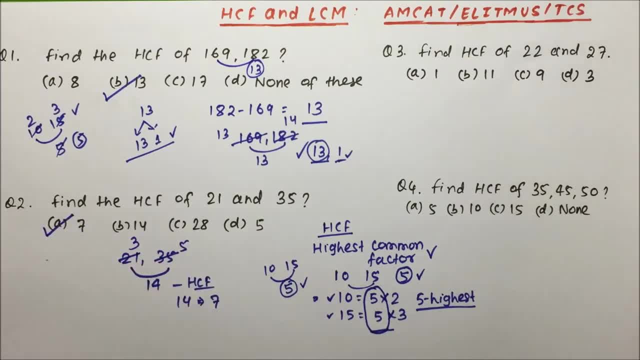 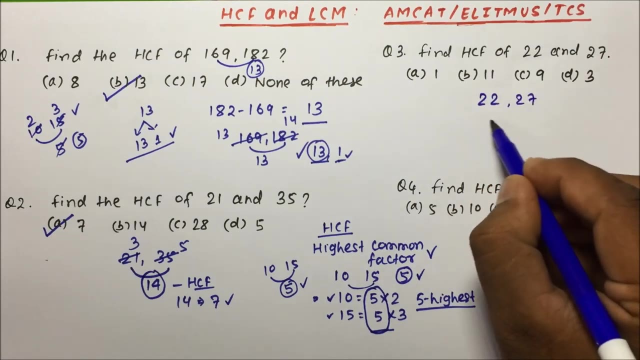 divide this by 5 times. That means 7 is the HCF, right, okay? So if you are not able to divide by the difference, then you take the next factor and then try to divide it. That will become our LCM, right, okay? Now find HCF of 22 and 27.. So, 22 and 27, you have to find out HCF. So take the. 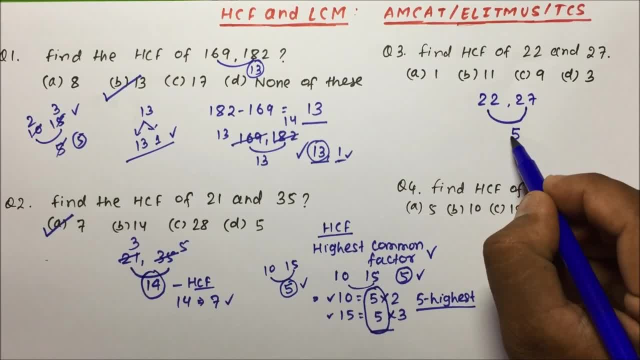 difference. So what will be the difference? The difference will be 5, right, okay, The difference will be 5.. But is this? numbers are divisible by 5? No, these numbers are not divisible by 5.. So 5, you will take factor. So 5 if you will divide by 1. So it will go by 5 times. So the second: 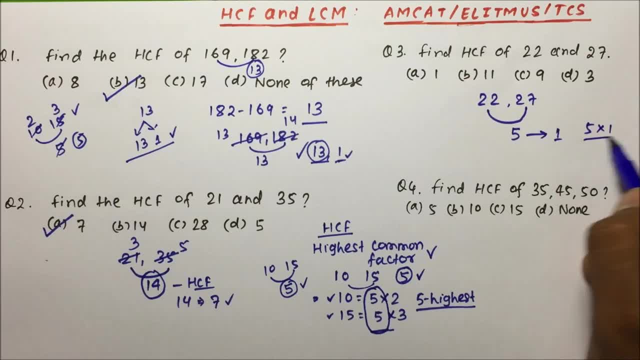 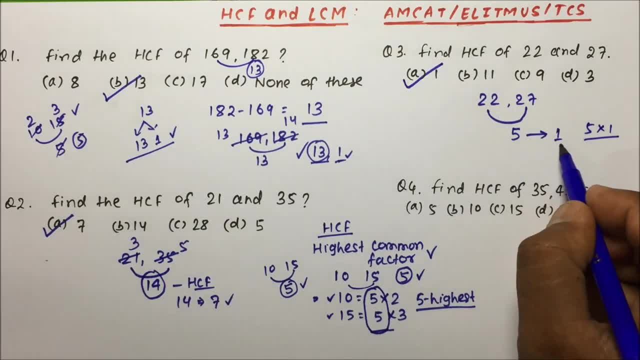 become option, A right okay, Because after 5 the next factor will be what 1.. So after 5 the next factor will be 1, because the factor of 5 is what 5 into 1.. Now we have 3 numbers here: 35,, 45 and 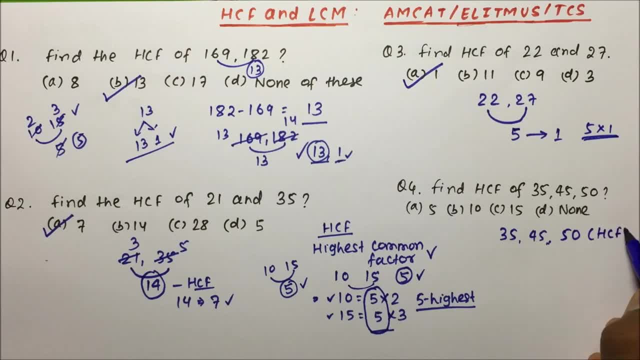 50. So this we have to calculate HCF. So how to calculate HCF of this? So if you want to calculate HCF of this, then you have to take the least difference. See least difference means what? 35 minus 45, right? okay, Take the positive value, This will be 10.. 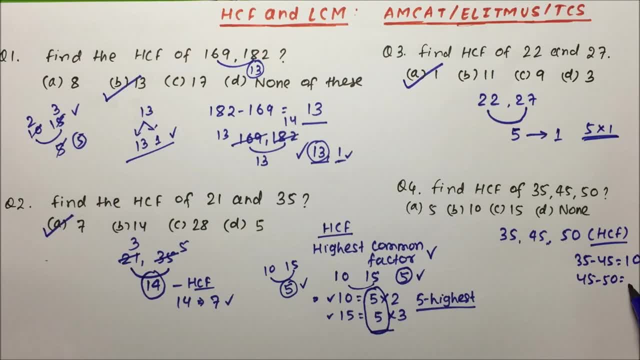 And then 45 minus 50. It will be what 5. And then you take 50 minus 35. It will be what 50. right? okay, See, friends, what I told. If you have 3 numbers and then if you have to calculate HCF, 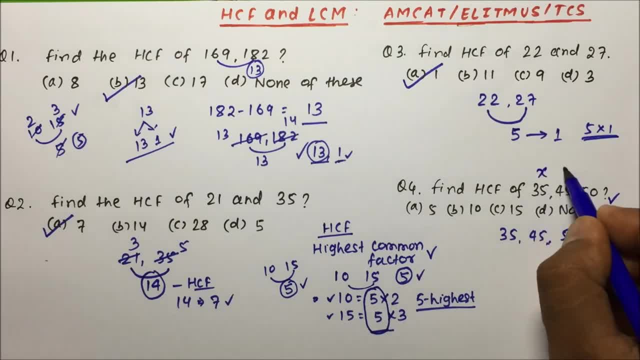 then how will you calculate? See, basically, the method will be there. Suppose: this is x, this is y and this is z. So it should be, it should be x minus y, and here modulus will be there, And then y minus z. modulus will be there, and then z minus x. right, okay So? 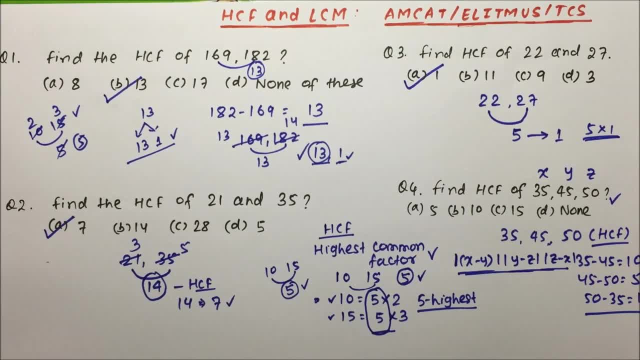 once we will get the difference, after that we will be able to calculate, right, okay, So let us see what will be the difference. So the difference, you see, the difference will be what? The difference will be 35 minus 45. The difference will be 10 and 45 minus 50. The difference will be 5. 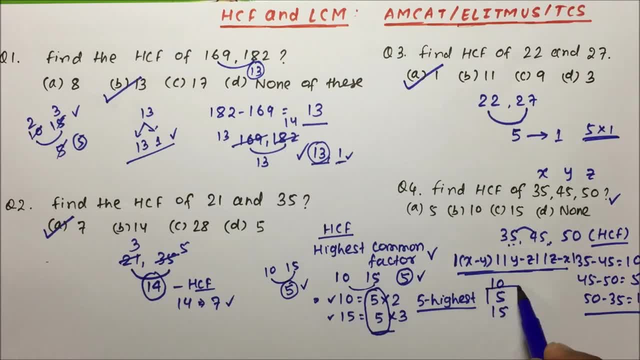 and 35 and 50 difference will be 15.. So you take the lowest number, So lowest number is what Lowest number is 5.. Now from 5 you try to divide this. So 5, 7, 5, 9 and 5, 10.. So 5 will be the. 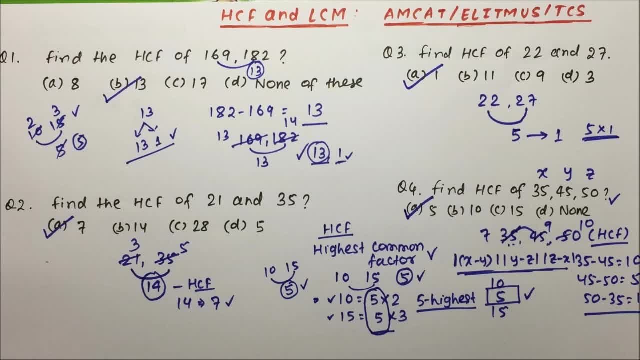 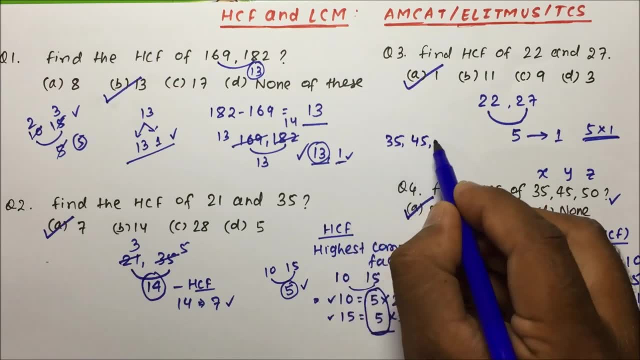 common factor of 35,, 45 and 50 right friends. So do not get confused. You know this question. we could have solved it in seconds, only because all these questions we are solving. all these questions we are solving without using pen and paper. So you see, the difference will be here: 10. The 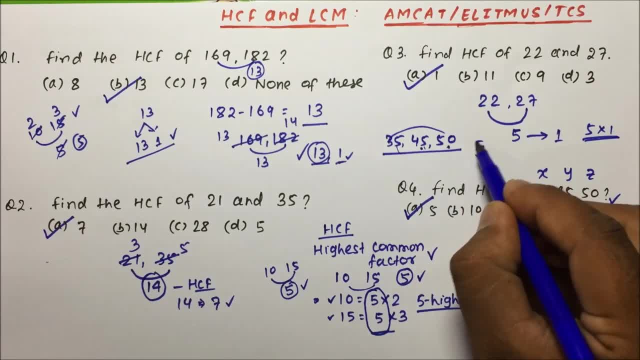 difference will be here 5 and the difference will be here 15.. So the least difference is 5, and 5 is able to divide all 3 numbers. That means my HCF is 5.. If 5 is not able to divide, then what? 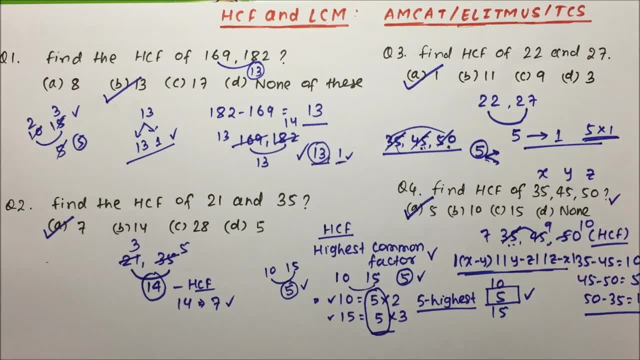 we will do. We will take the again factor of 5 and that will become our HCF right. okay, So all these 4 questions were very important and we are able to calculate the HCF in seconds. Let's move to the next part of HCF Now, question number 5.. We have 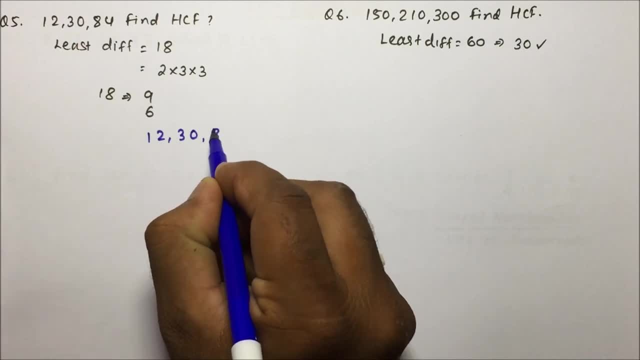 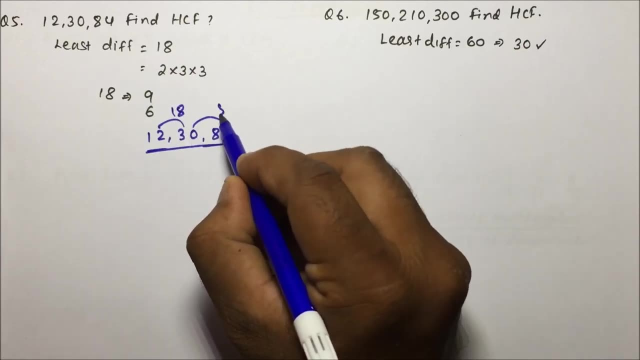 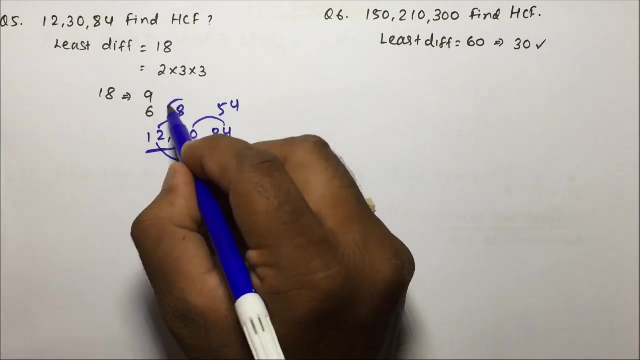 to find out the HCF of 12,, 30 and 84. right, okay, Now friends, find out the least difference, So least difference. this difference will be what 18.. This difference will be what 54 and this difference will be what 4 minus 2 is 2 and 8 minus 1 is 7.. So you have to take the least. 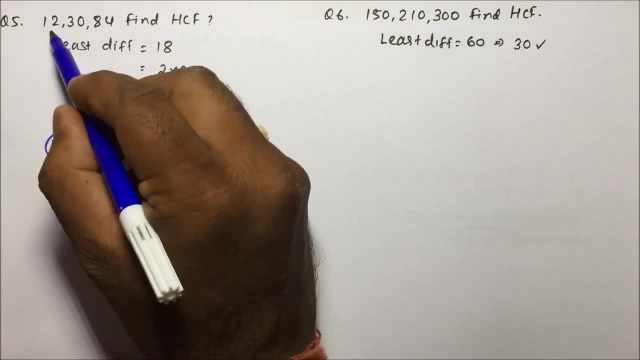 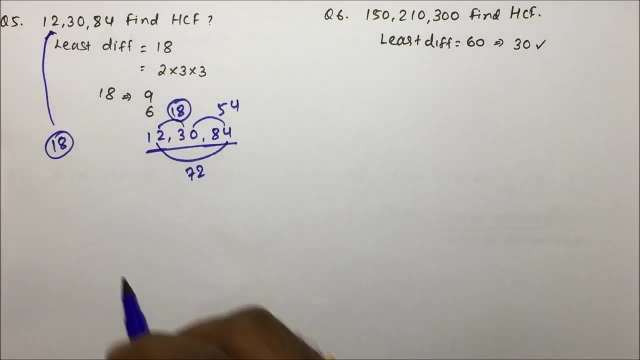 difference, So my least difference is 18.. So, from 18, from 18,, 12 is divisible, No. From 18,, 30 is divisible, No. From 18,, 84 is divisible, No, Right, okay. So friends, what we will do, We will factorize. 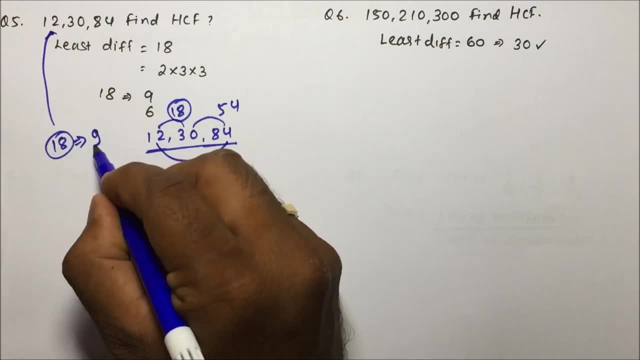 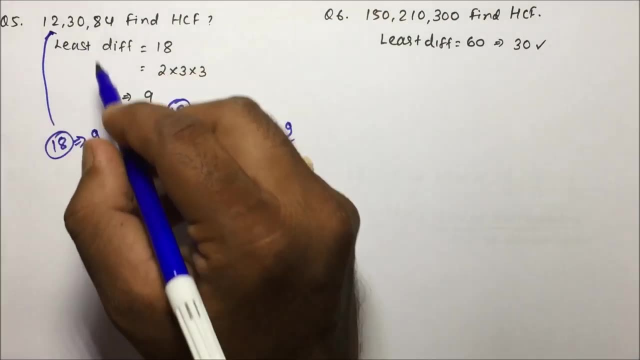 it. So what will be my next factor? If we will divide 18 by 2, it will go by 9 times. If we will divide 18 by 2, that will be my next factor. So next factor will be 9.. So from 9, 12 is divisible. 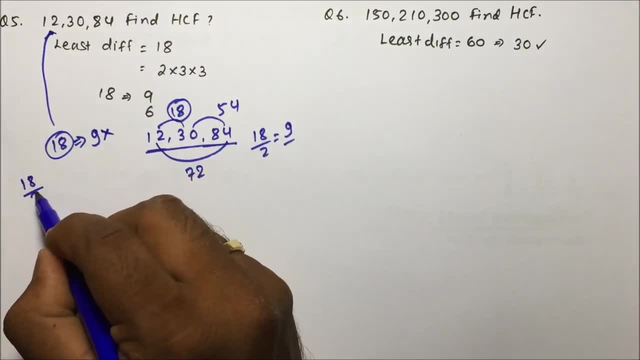 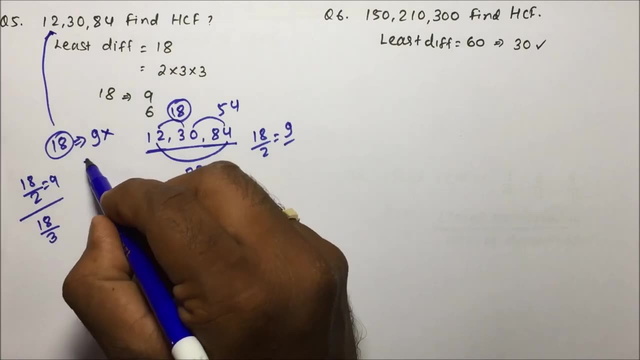 No, Then what will be the next factor, friends? So first we divided 18 by 2, then we got 9, but 9 is divisible. Then again we will divide 18 by 3.. So if we will divide 18 by 3, my next factor will be 6. 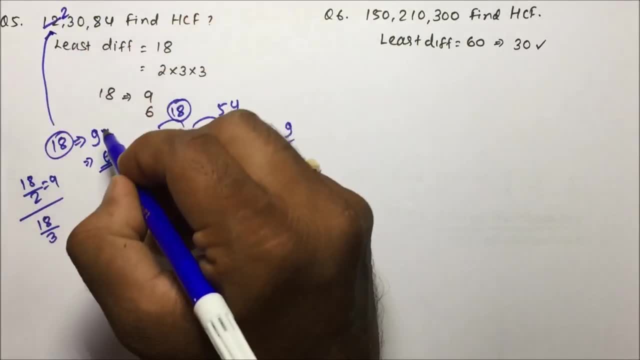 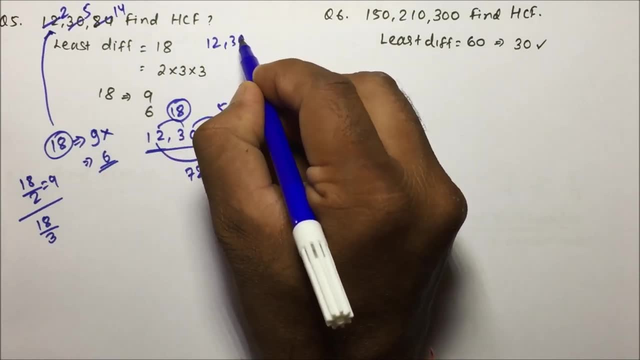 right, okay, My next factor will be 6.. Now, 6 will divide 12 by 2 times, 6 will divide 30 by 5 times and 6 will divide 84 by 14 times. That means a CF of 12, 30 and 84 will be what, friends? 6 right. 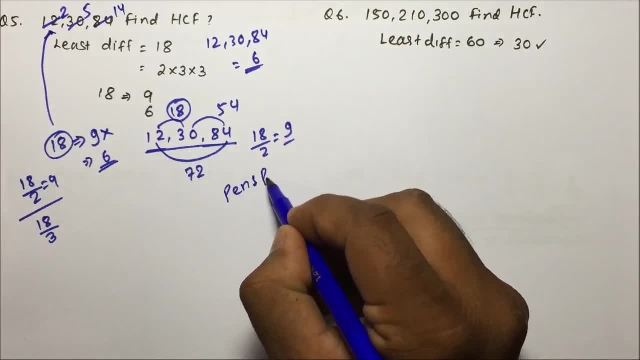 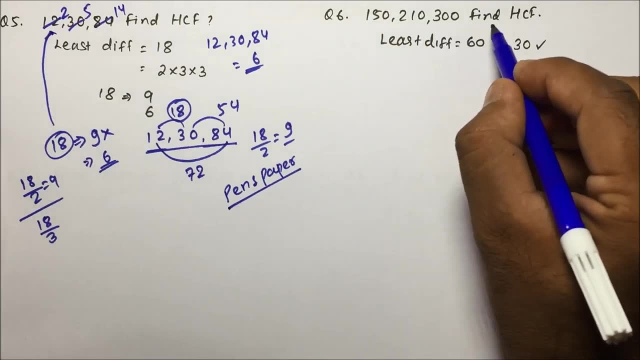 okay, So all these questions we can solve without pen and paper, friends, and in seconds, right okay? Next is find out the CF of 150,, 210 and 300, right Okay? So how will you find the CF? So what we will do? The first thing which we will do is we 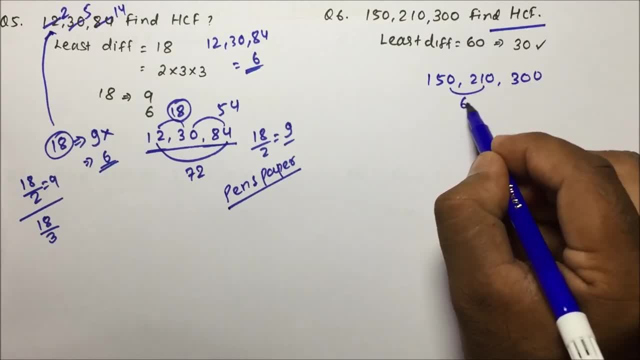 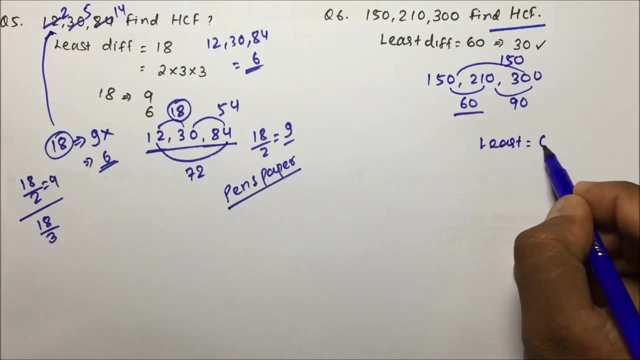 will take the difference. So let us see the difference. So this difference is what? This difference is 60.. This difference is 90 and this difference is 150, right, okay? So now the least difference is what, friends? The least difference is 60. But you see, 60 will not be able to divide. 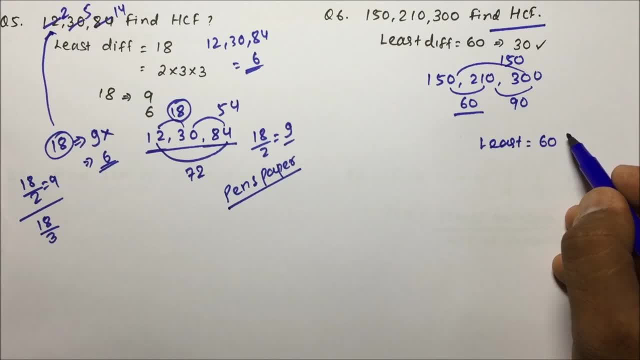 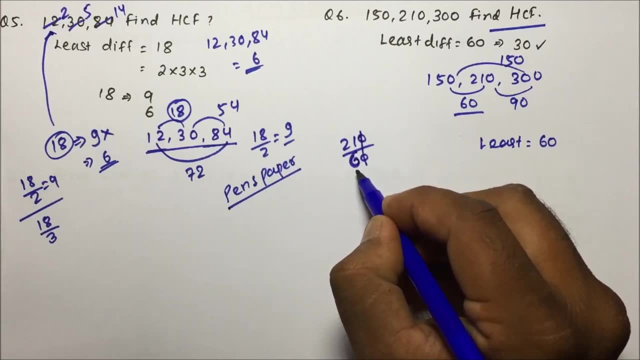 all those numbers here. right okay, 60 will not be able to divide all those numbers here. Basically, 60 will not be able to divide 210, right okay? 210 divided by 60. So it will not be able to divide it, right okay? 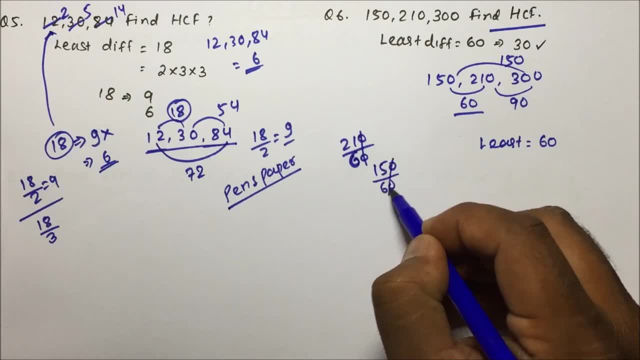 Even you can say 150 divided by 60. So 150 also will not be divisible by 60, right, okay? So what we will do? We will calculate the next factor. So next factor will be: what Divide 60 by 2.. 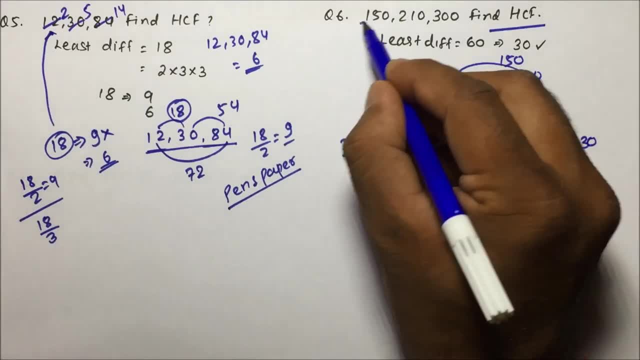 That will be 30.. That will be 30.. Now you see, 30 will be able to divide by 5 times, by 7 times and by 10 times. That means hcf of this number will be what Equal to 30.. 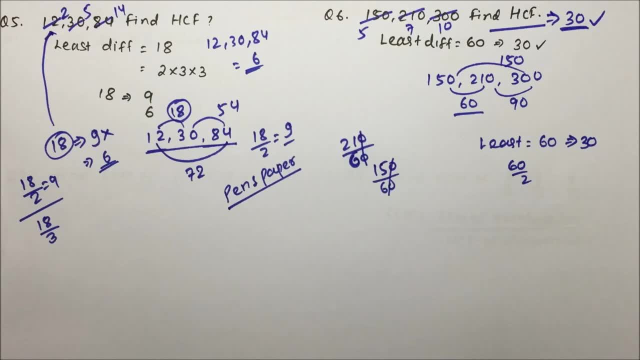 So I hope you would have understood how to calculate hcf. Now let's move to LCM. right okay? So you have to find out LCM of this number, right okay? So let's understand what is LCM. 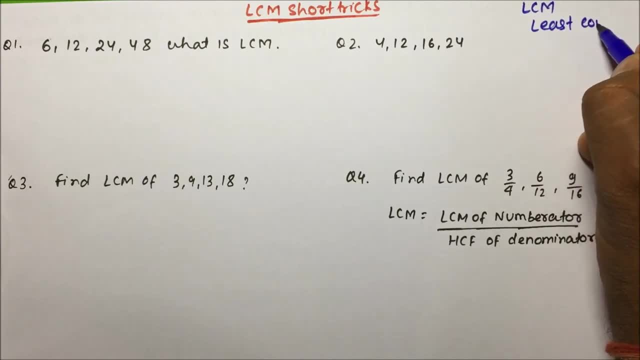 So LCM is nothing but least common multiple. LCM is nothing but least common multiple, or they can also say lowest common factor. right okay, Both are same. Now suppose if you have 4 and suppose if you have 2, right okay? 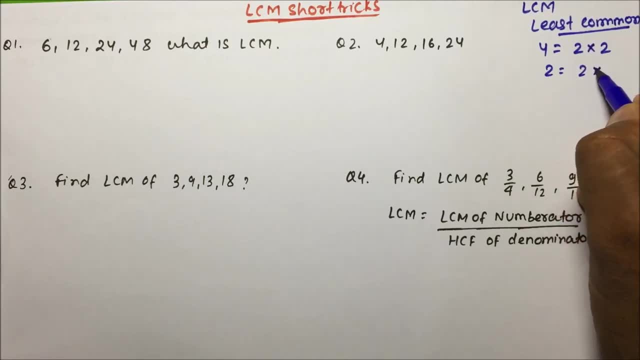 So you will see 4, how will you write 2 into 2 and 2, how will you write 2 into 1, right, okay? So if I will ask you what is the least common factor? right, okay? 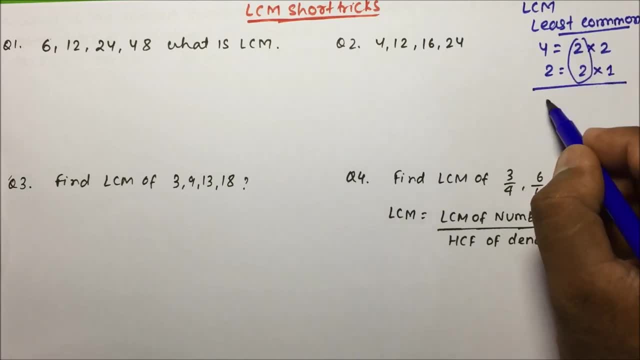 So what is the least value which is common in both, so which is nothing but 2,, right, okay? So if I will tell you So, if it is 16 and if it is 32, then it will be 2 into 2 into 2, something like that, right. 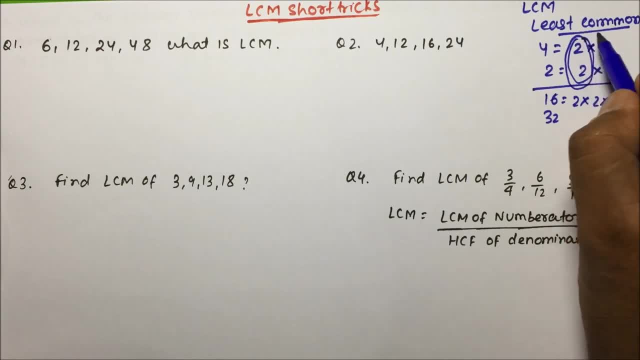 okay. So basically what you have to do, you have to find out the least common- See the meaning of LCM- is least common, multiple. So what is the least value which is multiple in both? right, okay, Now let's see how we are going to calculate the LCM in seconds. 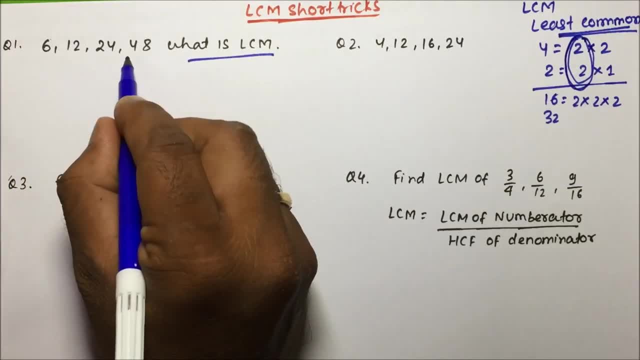 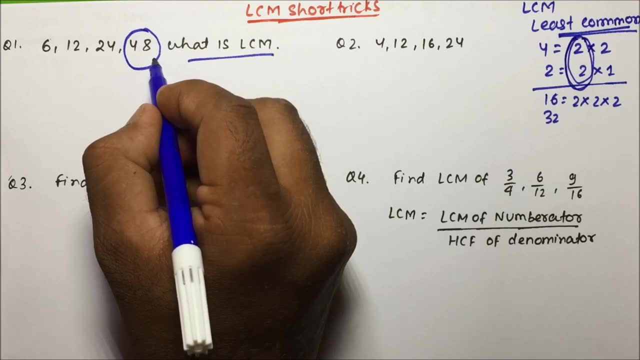 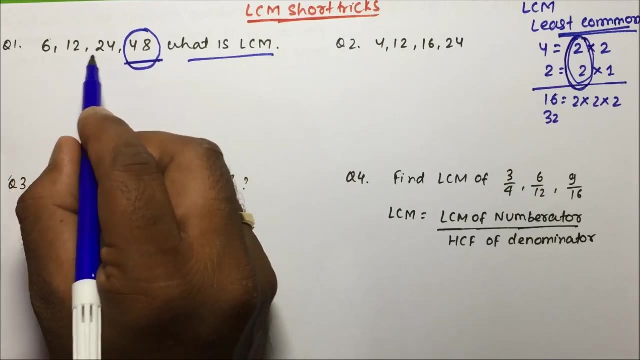 So basically, you have to calculate the LCM of 6, 12, 24 and 48. So what is the biggest number here? What is the largest number here? So the largest number here is 48.. Now, is this largest number? is this bigger number? is divisible by 6, 12 and 24?? 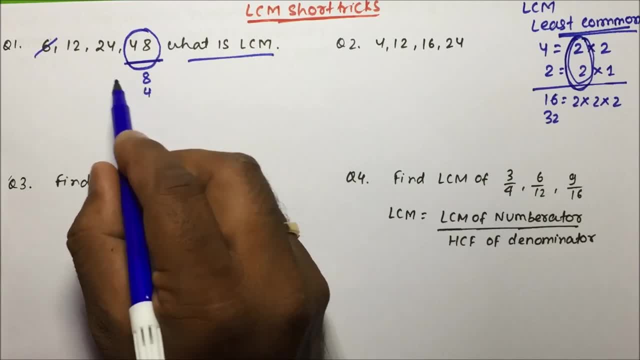 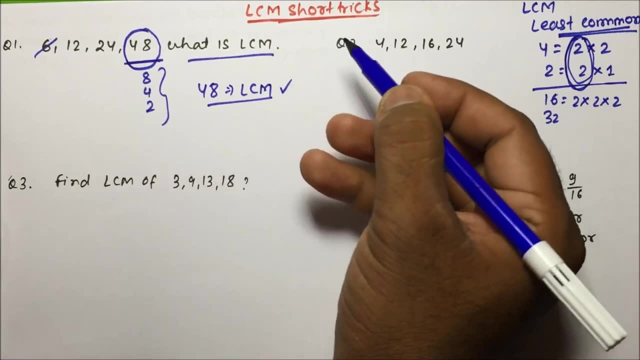 Yes, 6 will divide this by 8 times, 12 will divide this by 4 times and 24 will divide this by 2 times. that means 48 is nothing but LCM. that means 48 is nothing but the LCM right okay. 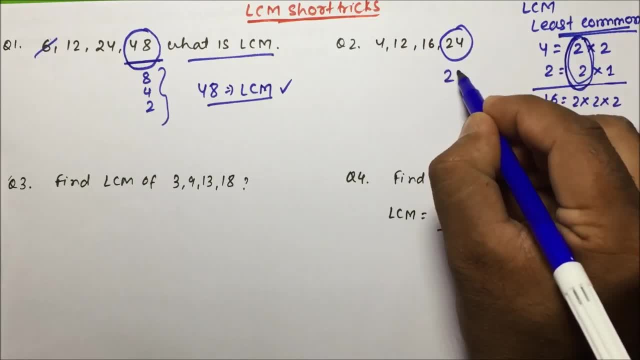 So pick the largest number, pick the bigger number, So you can say: bigger number is what here? 24, right, okay, 24 is divisible by 4,, 24 is divisible by 12, but 24 is not divisible by 16,, right. 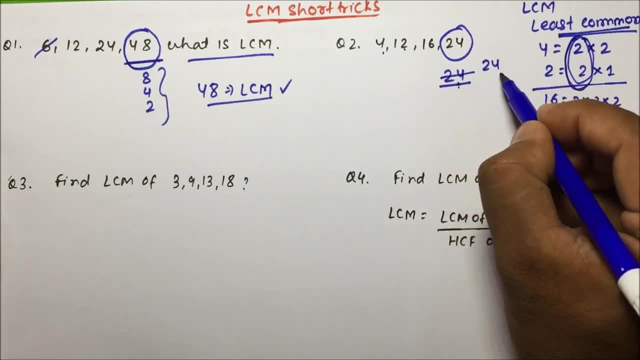 okay, So take the next number. So next number, 24- factor will be what 24 into 1 is 24 and the next factor of 24 will be what 48.. Next factor will be what 48.. 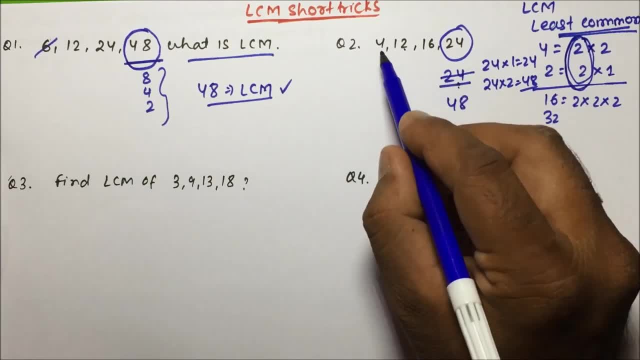 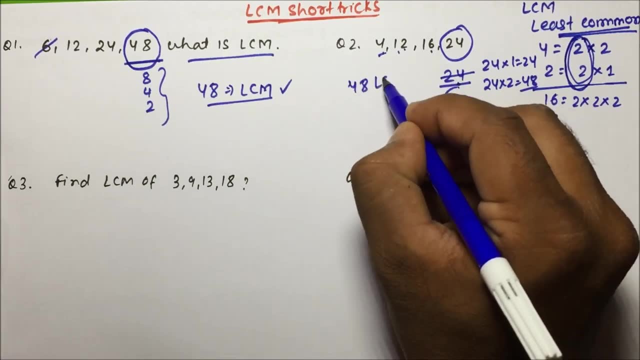 So now you can see, the next factor will be 48.. Now you see, 48 is divisible by 4, yes. 48 is divisible by 12, yes. 48 is divisible by 16, yes. So 48 will be again LCM of this question as well, right, okay? 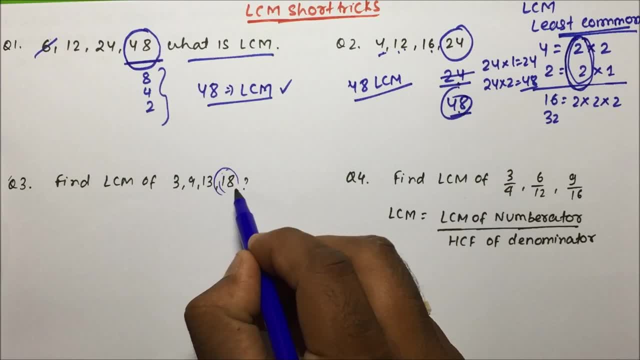 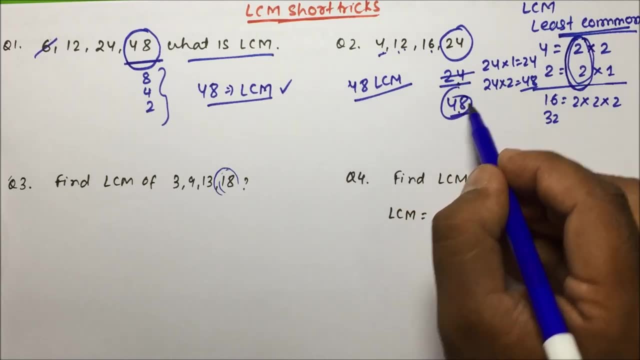 So what you have to do, You have to pick the bigger number. You have to pick the bigger number and then you have to see if it is Getting divisible by the other number. Otherwise you have to take the next multiple of that, right, okay? 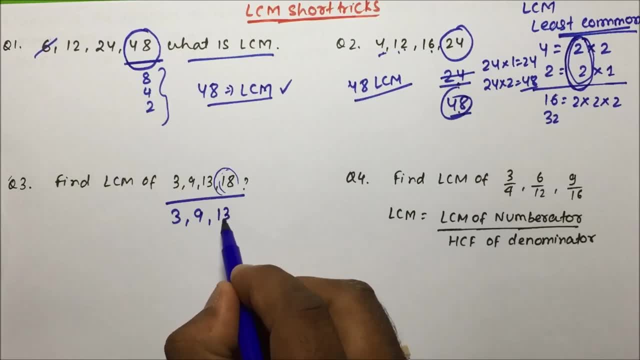 Now, here you see, we have 3,, 9,, 13 and 18.. See, 13 is a prime number, 13 is a prime number, right, okay? So, except 13,, you can see 18 is divisible by 9 and 3,, right, okay? 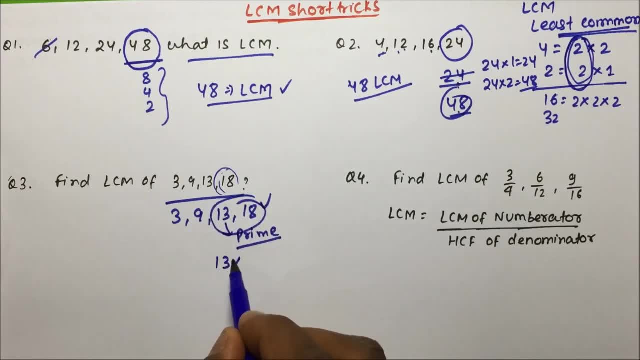 So if you have any prime number, then what you have to do You have to multiply 13 and 18.. And whatever multiplication comes, 13 into 10 is 130 and 13 into 8 is what- 104.. 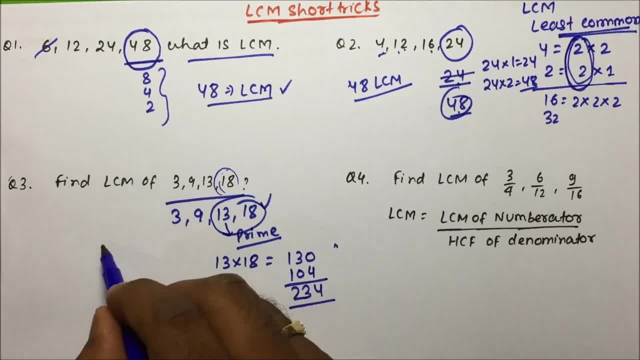 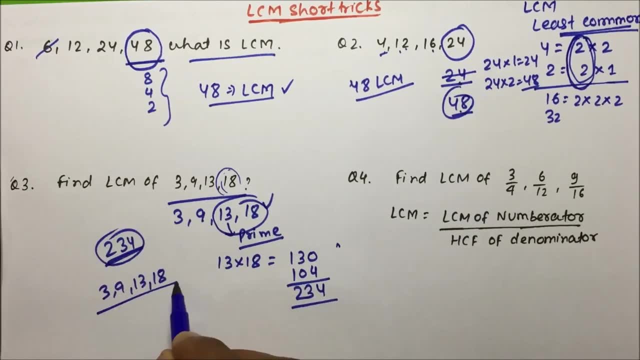 13 into 8 will be Okay: 104, 3, 2.. That means 234 will be the LCM of 3,, 3,, 9,, 13 and 18.. 3,, 9,, 13 and 18 because the reason is the reason is there is a prime number, is there? 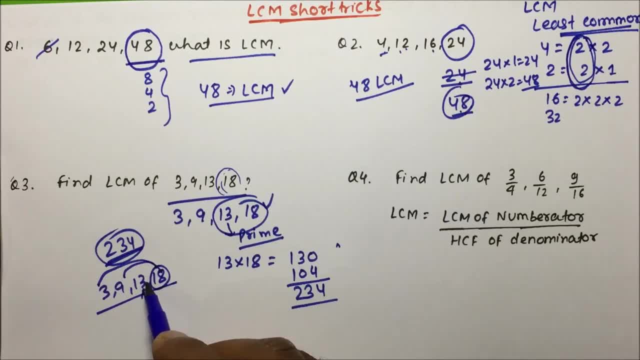 See: 18 is divisible by 9 and 13.. But 18 will be divisible by this prime number only when we will calculate 18 into 13,. right, okay, So hope this will be clear Now. the next LCM which you have to calculate is for fraction. 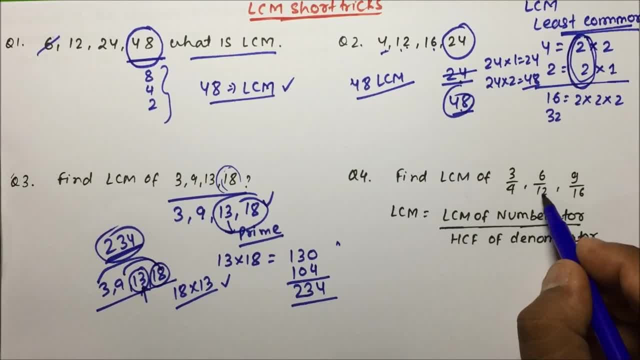 The next LCM which you have to calculate is therefore the fraction, So 3 by 4,, 6 by 12 and 9 by 16, you have to calculate the LCM. So LCM will be, LCM will be LCM of numerator divided by SCF of denominator right. okay. 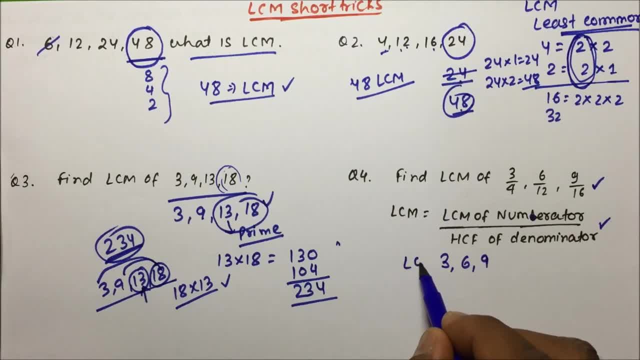 So, basically what you have to do, you have to calculate LCM of 3,, 6,, 9, right, okay. And then you have to calculate SCF of denominator, means 4,, 12 and 16.. So LCM of this number will be what? 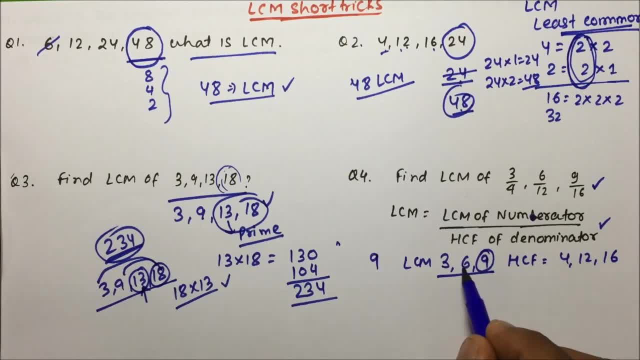 See 9.. What is the maximum number value? Maximum value is 9.. But 9 is not divisible by 16.. So what we will do? We will take the next number, 18.. 18 is divisible by 3 also. 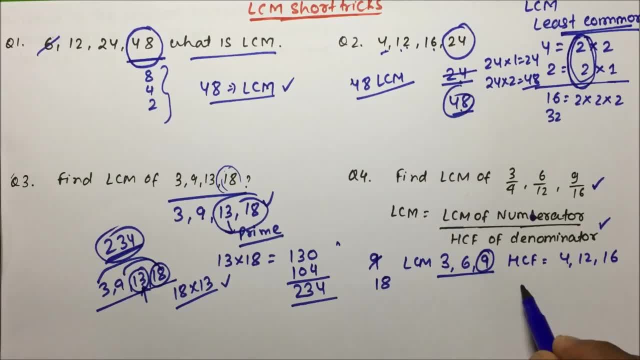 18 is divisible by 6. also, That means LCM will become LCM will become 18.. And what about SCF? SCF, you will see, the difference will be 8 and the difference will be 4.. Now, 4 is able to divide all 3.. 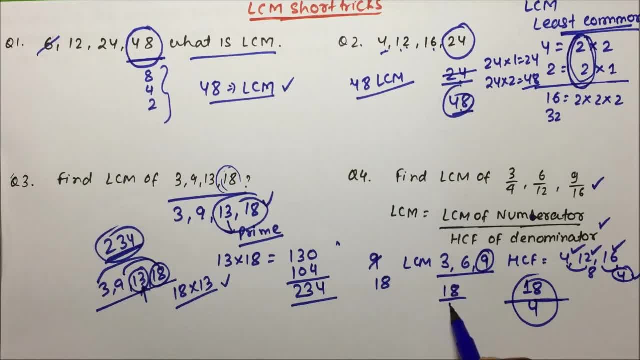 That means SCF will become 4.. So 18 by 4 will be the LCM, or you can say 9 by 2 will be the LCM of 9 by 2 will be the LCM of 3 by 4,, 6 by 12 and 9 by 16.. 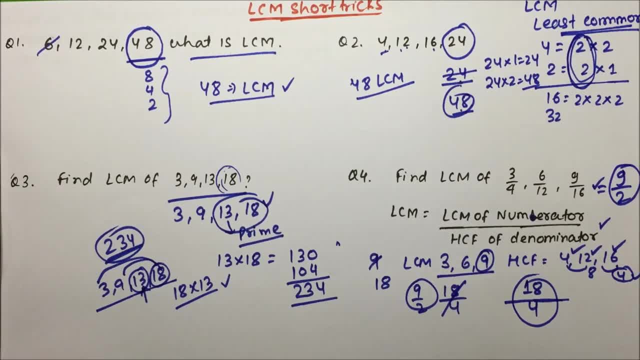 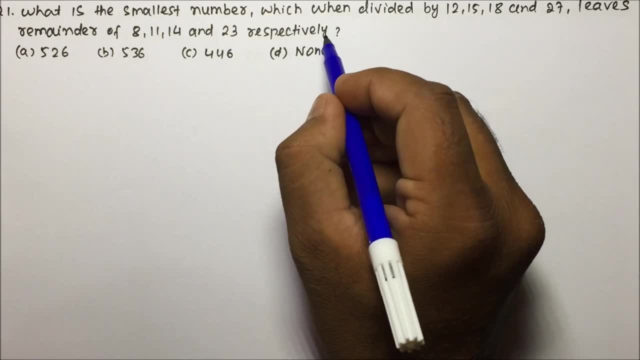 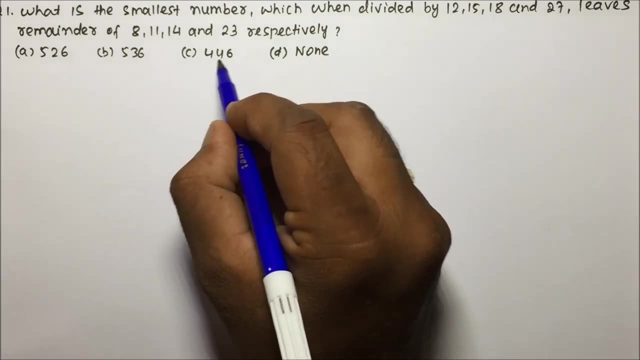 So hope you would have understood the LCM as well. Now we are moving towards the type of Questions which comes in your exam, So let's start with the question number 1.. So question number 1 is: what is the smallest number which, when divided by 12, 15,, 18 and 27, leaves remainder of 8,, 11,, 14 and 23.. 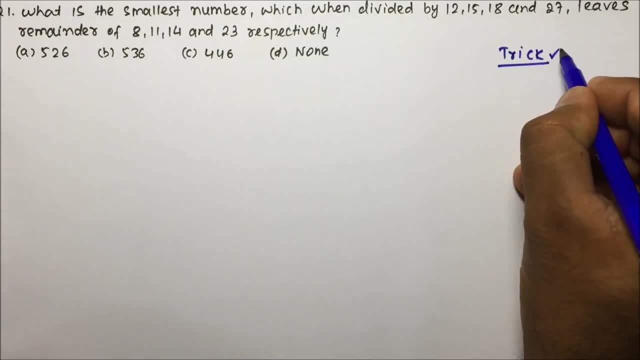 See, there is a trick here, So that trick only you have to apply on this kind of question, right, Okay? So what is the smallest number? So a smallest number will be always your LCM. So a smallest number will be always your LCM. 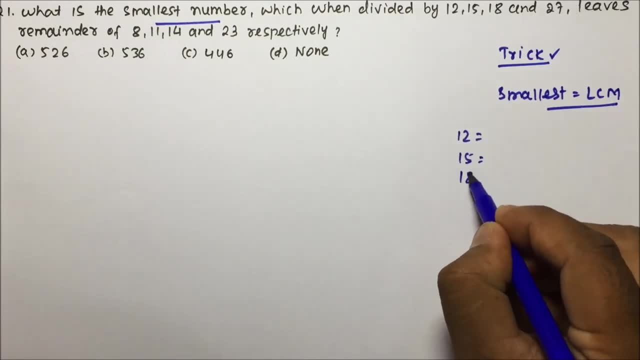 So let's take LCM of 12.. 15.. 18 and 27.. So I am going to teach you a different method here to take LCM: See 12. I can write 2 into 2 into 3.. 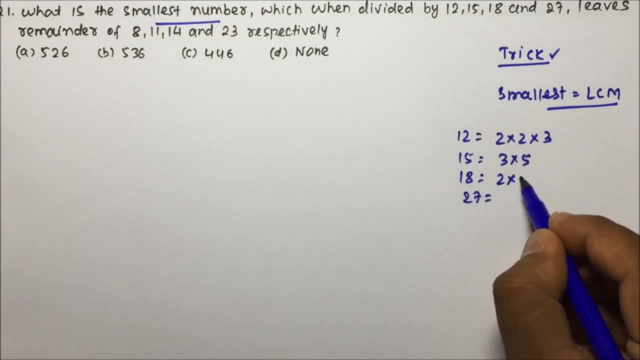 15: I can write 3 into 5.. 18: I can write 2 into 3, 6.. 6 into 3 is 18.. 27: I can write 3 into 3 into 3, right, Okay. 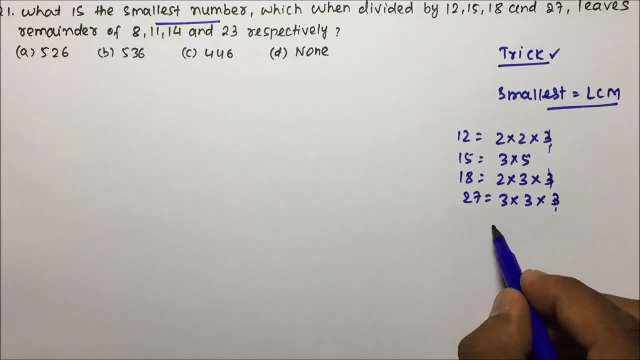 Now you see these 3 are common in all 3.. So instead of all 3, you write 1, 3. Then you see 5 is alone, So 5 you write here. Okay, Then you see these 2 is common in both, right. 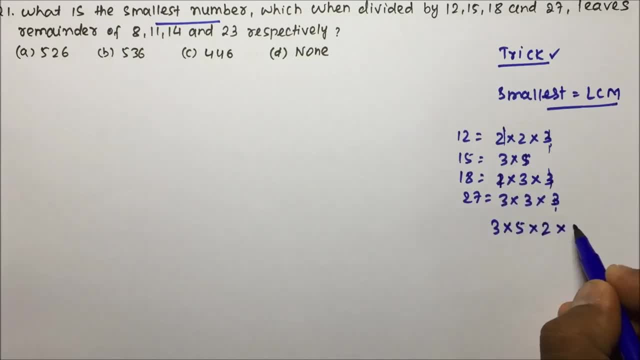 Okay, These 2 is common in both. It is not common in any other. So write 2 here, Then you see these 3 are common in both, 3, 3.. So write 1 more 3 here. 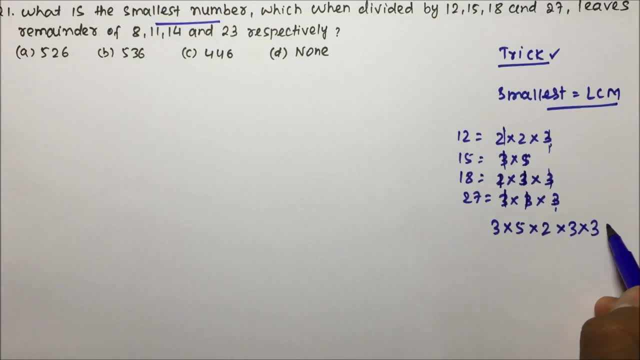 And then you see these 2, 3 are common in both. Write 1 more 3 here And then 1, 2 is remaining. So you write 2 here Now. 5 into 2 will be 10.. 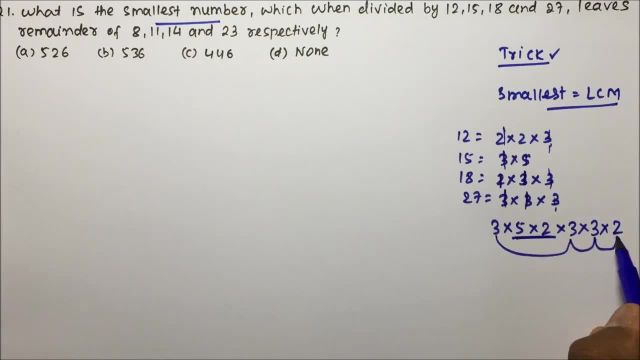 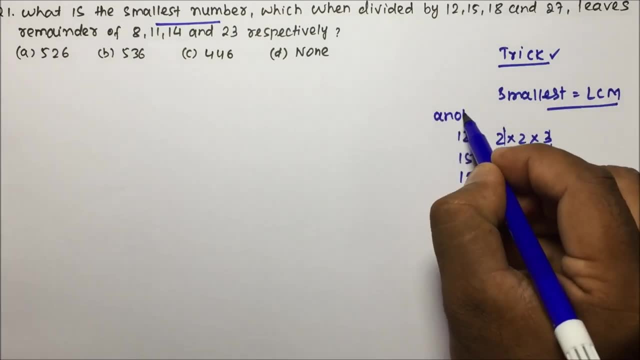 So 3 into 3 is 9.. 9 into 3 is 27.. 27 into 2 is 54. And 54 into 10 will be 540.. So this is one another method. This is one another method where we will be able to take the LCM. 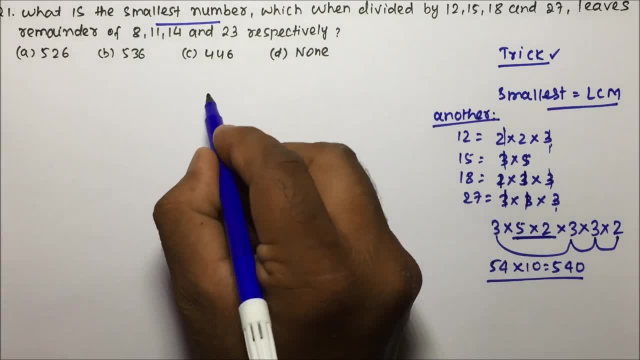 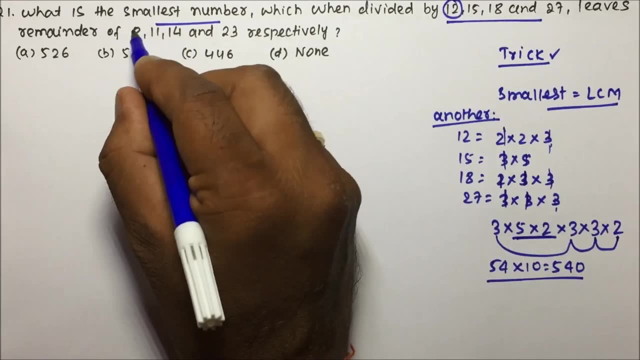 Very much easily, Right Okay, So LCM of this number will become LCM of this number will become 540.. Right, Okay, Now you see the difference. So difference is what See here: 12 and 8.. 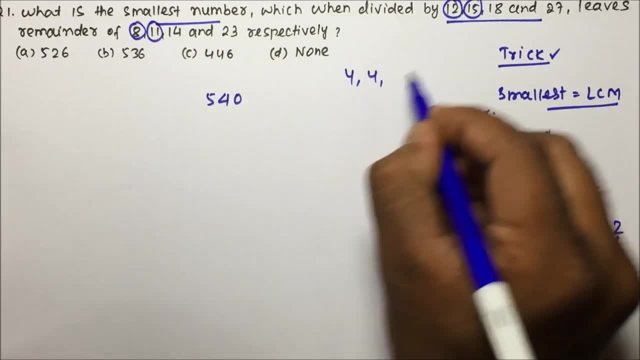 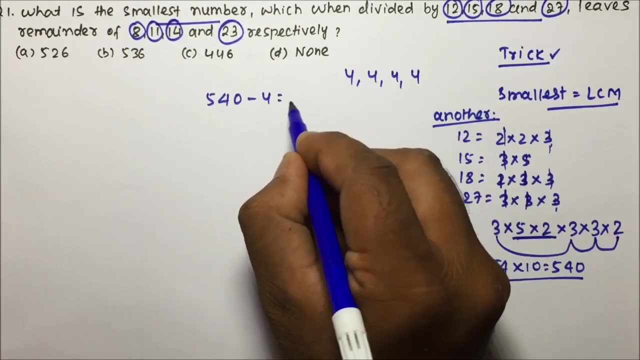 The difference is 4. 15 and 11.. The difference is 4. 18 and 14.. The difference is 4. 27 and 23.. The difference is 4.. So subtract 4 from this, You will get 536.. 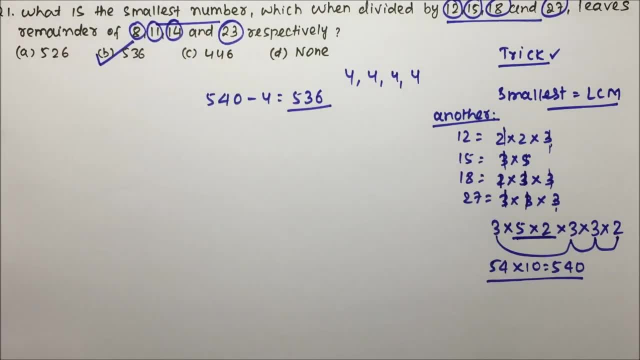 That means option B will be the correct answer for this question. See what I did here. What is the smallest number? What is the smallest number? What is the smallest number If they are telling you a smallest number? that is nothing but LCM. 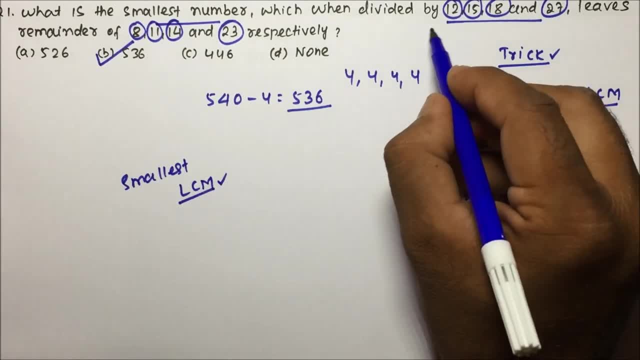 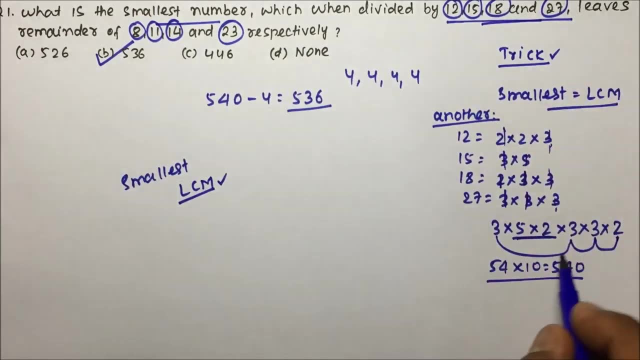 And if they are telling you the largest number, that is nothing but HCF, So which, when divided by 12,, 15,, 18 and 27, leaves remainder of this Right. Okay, So first calculate the LCM. 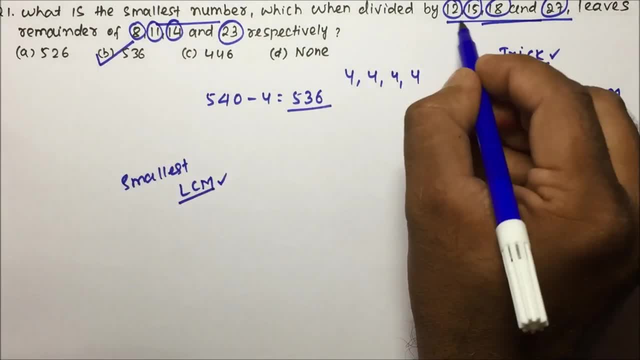 So LCM is 540.. Right, Okay, And then see the difference. So the difference is 4, 4,, 4, 4.. That means subtract 4 from that, 536 will be the smallest number. 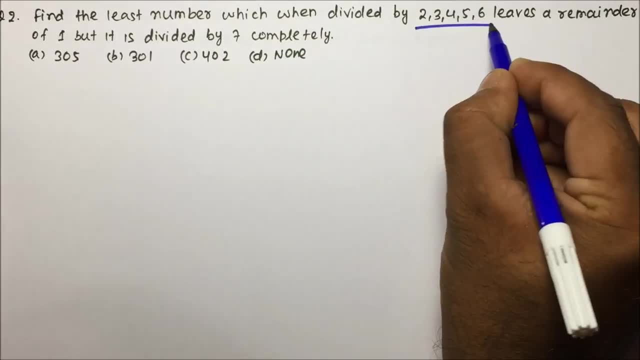 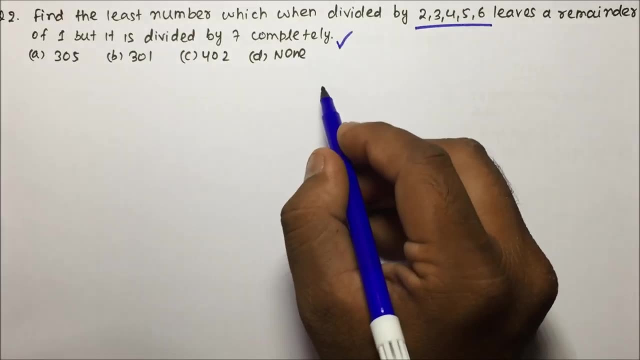 Option number 2 is find the least number which, when divided by 23456, leaves a remainder of 1, but it is divided by 7, completely Right, Okay, So you have to find the least number. See. least number is nothing, but whenever the least number is there, whenever the 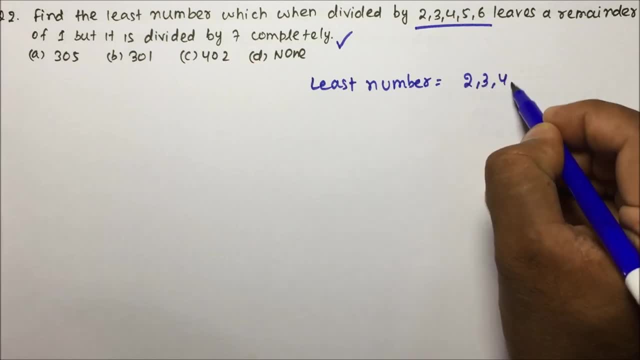 smallest number is there. you have to find the LCM. So LCM of 23456.. So what will be the LCM? See, you can see, 6 is not divisible by everything. Right, Okay, 6 is not divisible by everything. 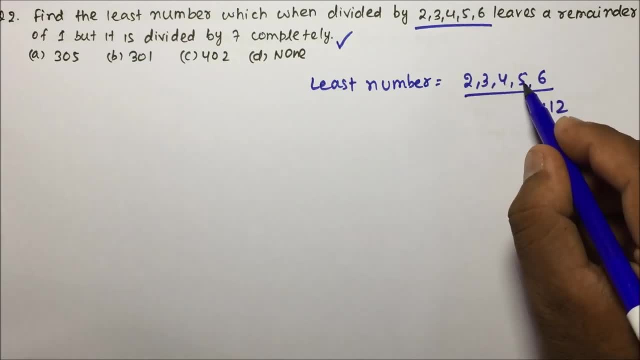 Then what we will do. We'll take the next factor of 6.. So 6, 12.. 12 is again not divisible by 5.. Then again what we will do. We will take third one, So the third factor. 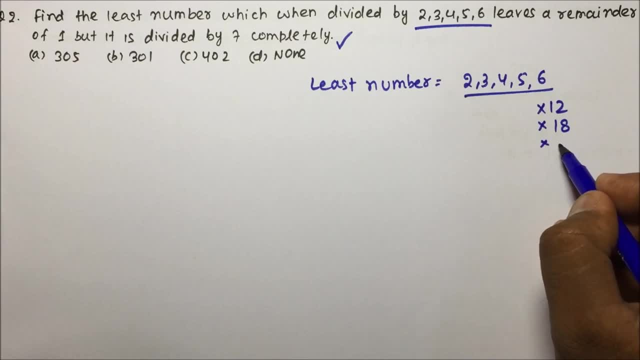 It will be 18.. Again, 18 is not divisible by 5.. Then we will take fourth, 24.. Then we will take 30. See basically what will happen. if 5 is there, then 0 should be at the end, or 5. 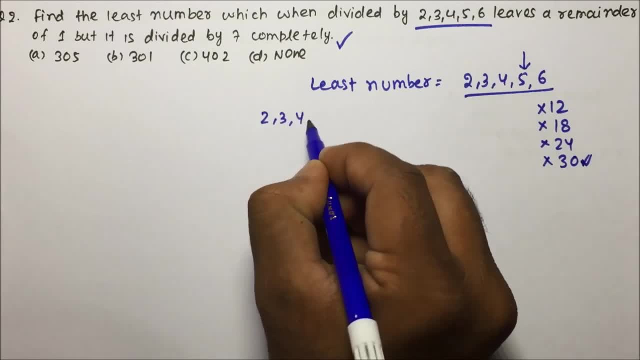 should be at the end, Right Okay? See, if I ask you to friends calculate the LCM of this number, then you can see the LCM of this number has to be the factor of the maximum value, Right Okay. 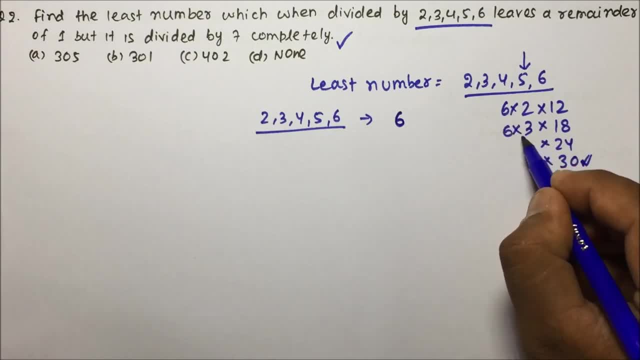 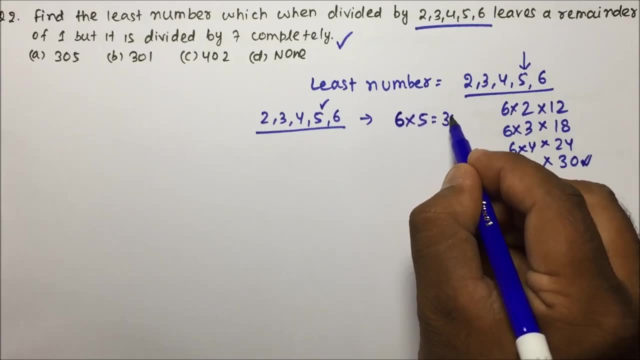 So I cannot, you know, simply take 6 into 3,, 6 into 2,, 6 into 4.. Right Okay, Because this number has to be divisible by 5. also Right Okay, So that number, either I can take 6 into 5.. 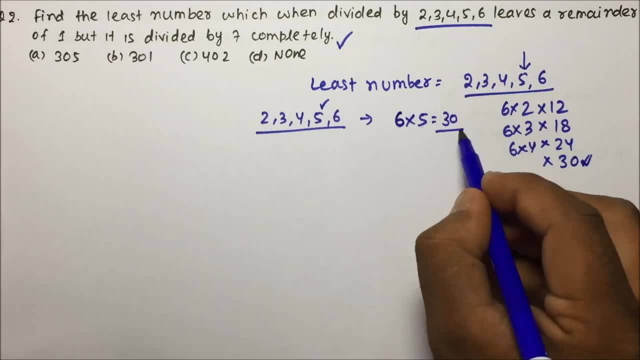 6 into 5 will be what 30. But 30 will not be divisible by 4. So 30 cannot be the LCM. The next number, if I will take the next number, will be 6 into 10.. 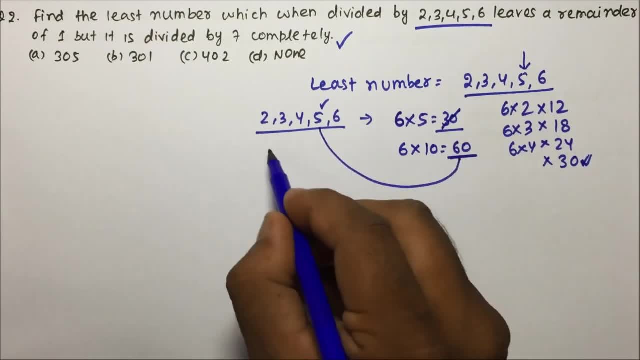 60.. Right, Okay, So you can see 60 will be divisible by 5.. Right, Okay, So 60 is divisible by 2. also, 60 is divisible by 3. also 60 is divisible by 4 also. 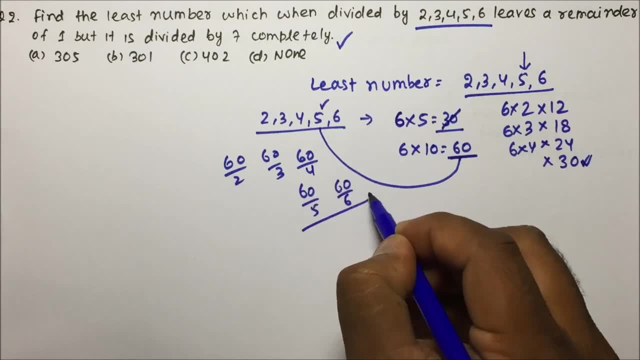 60 is divisible by 5 also, And 60 is divisible by 6 also, Right Okay? So you can see here the LCM will be equal to what? LCM will be equal to 60. Right, Okay. 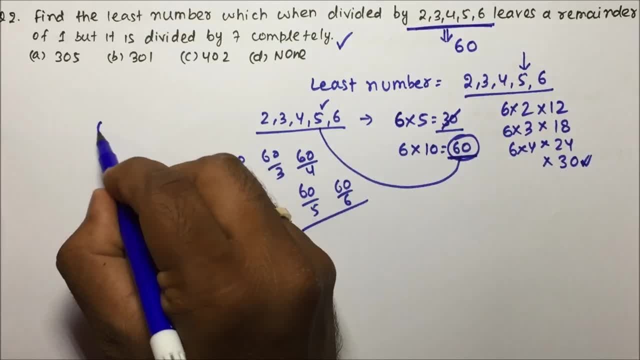 So here, LCM, I calculated because I am talking about the least number. So the least number is 60.. Right, Okay, So if the LCM is 60, if the least number is 60, that means 60 will be divisible completely. 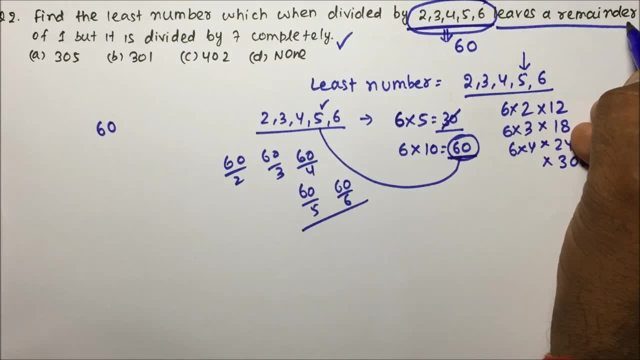 by all this number. But here they are telling they are leaving a remainder of 1.. They are leaving a remainder of 1.. So make this 61. So make this 60 plus 1, 61. Now 61. if you will try to divide it by 2 times, then it will go by 30 times. 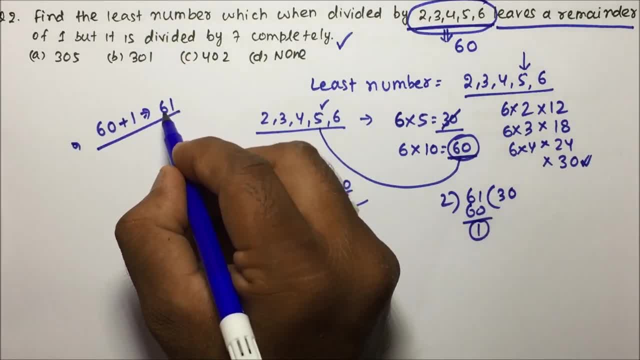 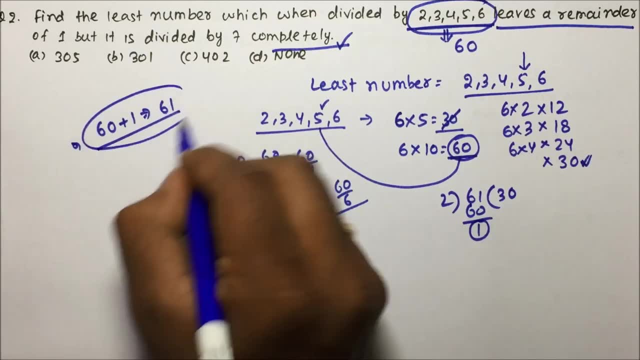 So 1 will be remainder. Then 1 will be remainder, Right Okay. Now what they are telling? It leaves a remainder of 1, but it is divisible by 7, completely Right Okay. So if the number has to be divisible by 7, then see 61. what can I write? 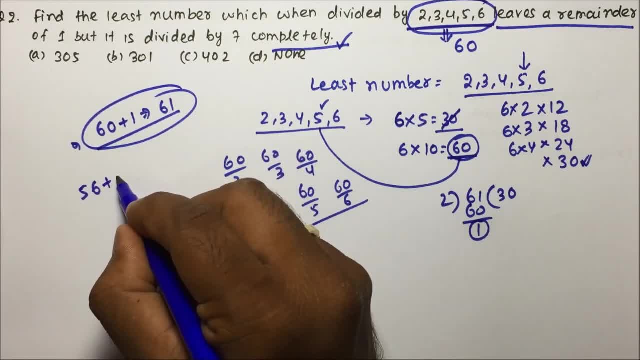 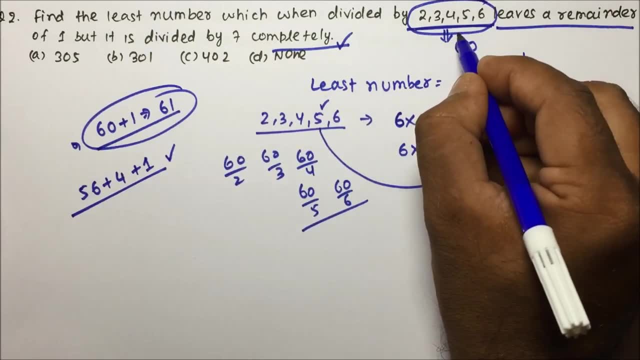 61. I can write 56 plus 56 plus 4 plus 1.. Right, Okay, This will be 61.. Right, Okay, See, 61 is a least number which will be divisible by all this number and leaves a remainder. 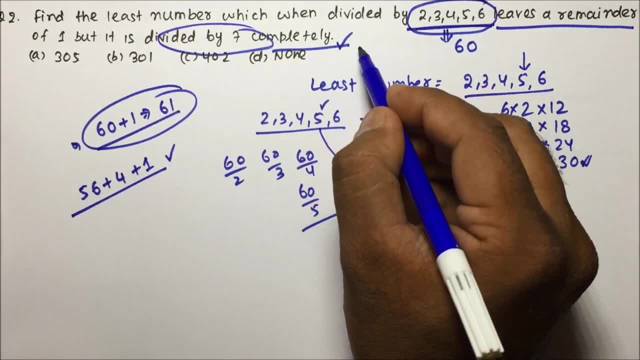 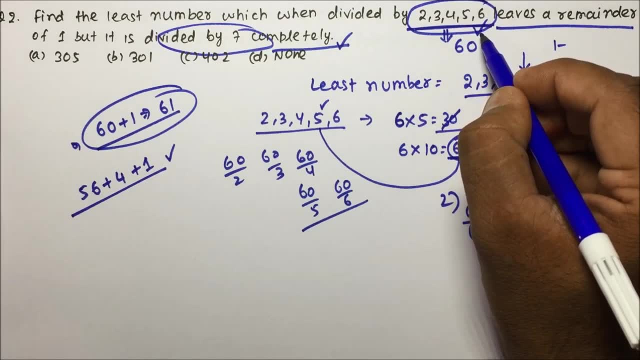 of 1.. But what they are asking? It should be completely divisible by 7. also, Conditions are same. Conditions are there. See, the first condition is it should be divisible by all these numbers, Right, Okay, Because this is a LCM of this number. 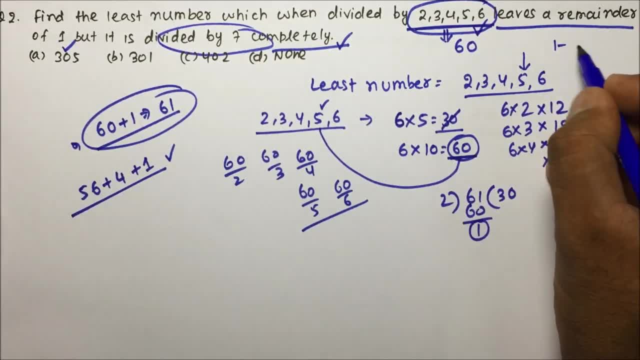 Right, Okay, And the remainder should be 1.. And the second condition is: see, 61 is a least number, which is which is, you know, divided by, which is divided by all those numbers, and it will give a remainder of 1.. 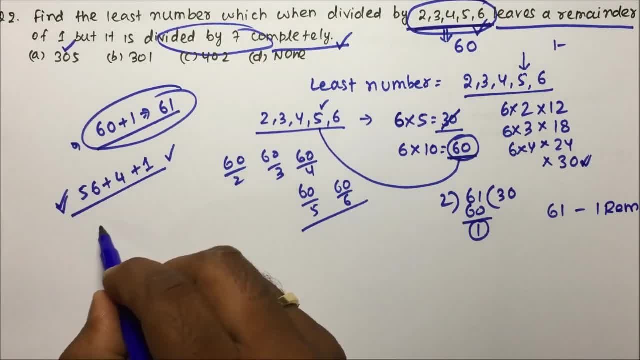 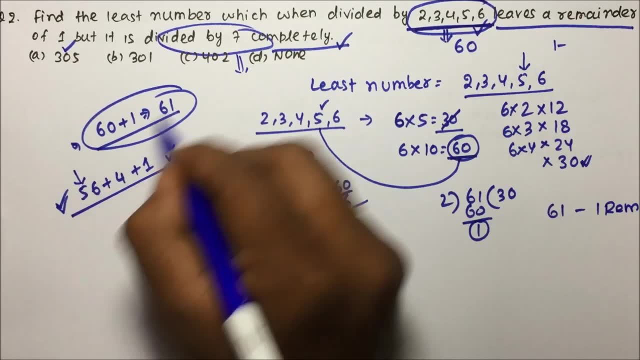 But it should be divisible by 7 also. So that number, basically we have to find it out and that is a challenge. Right, Okay, Now 61. I can write 56 plus 4 plus 1.. Why 56?? 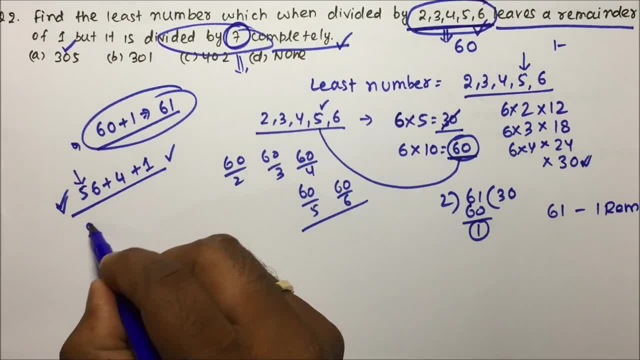 Because I am searching a number which is divisible by 7.. Now, 56, I can write 56. I can write 56k plus 4k plus 1.. See why I am assuming k here, because I do not know what the what will be the value. 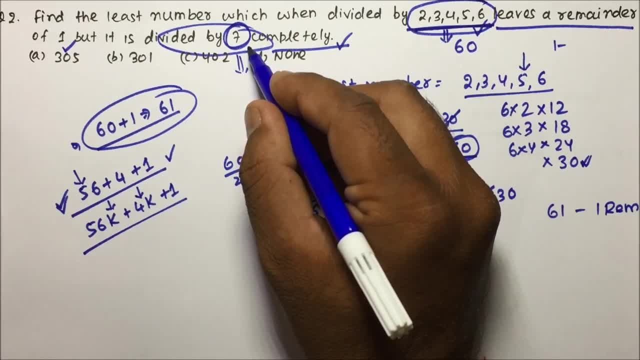 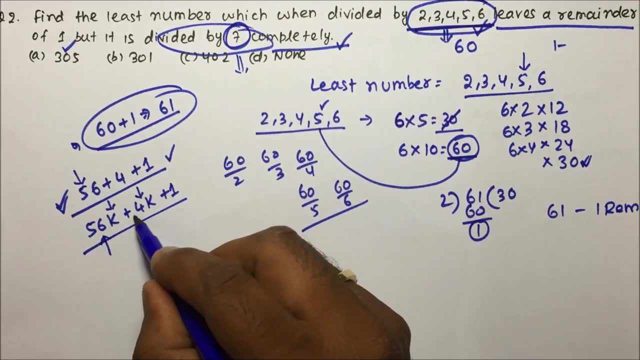 of k and so that this number will become- this number will become- divisible by 7.. Right, Okay, But I know 56. whatever the value of k is there, it will be divisible by 7.. Now we have to look for this number. 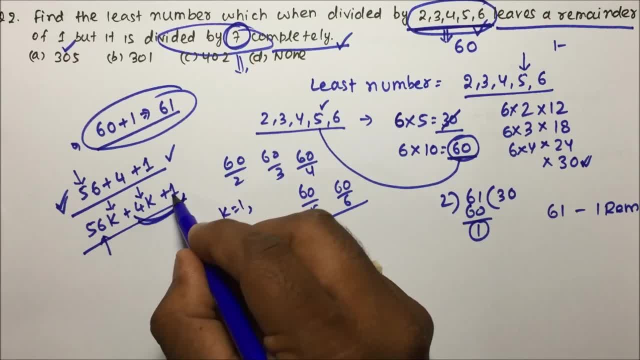 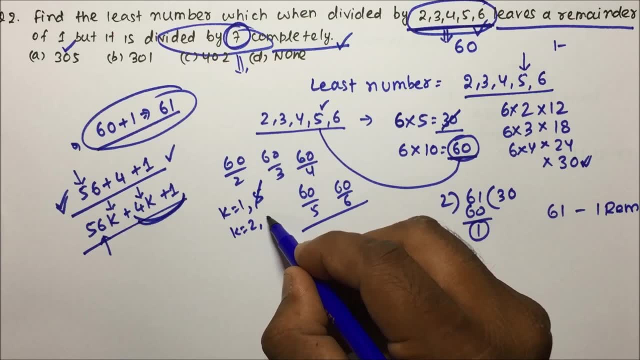 So k value I am taking 1.. If I will take the value of k is equals to 1, then 4 plus 1 will become 5, 5 is not divisible by 7.. k value 2, then 4 into 2 is 8 plus 1, not divisible by 7.. 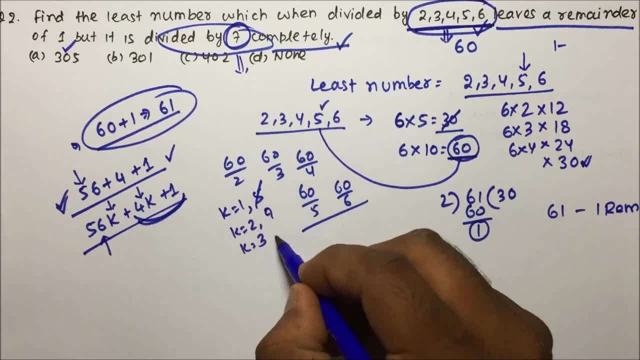 Right, Okay, Then k is equals to 3. So 4 into 3 plus 1,, 13.. 13 is again not divisible by 7.. k is equals to 4. So 4 into 4 plus 1,. 17 is again not divisible by 7.. 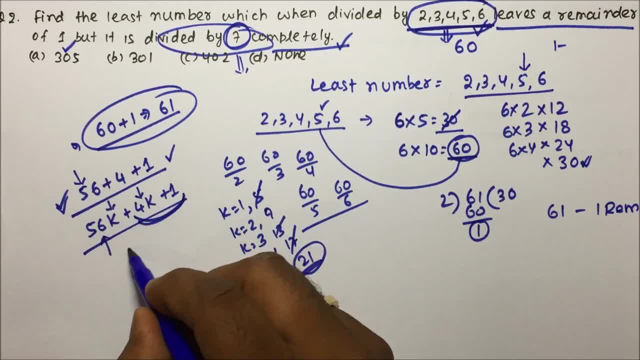 Then k is equals to 5.. Then it will become 21.. So for the k is equals to 5, this number will be divisible by 7.. So 56 into 5 plus 1.. 56 plus 4 into 5 plus 1.. 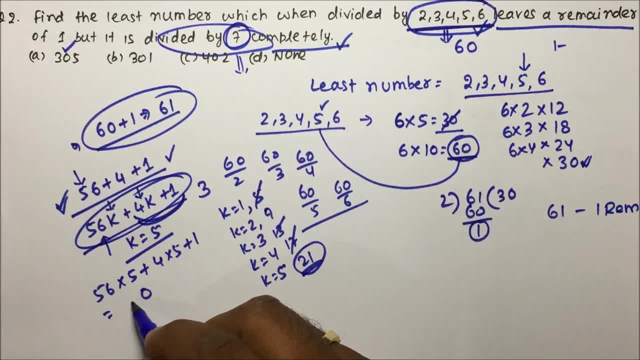 If you multiply 5 into 6 is 30 and 25,, 5 into 6 is 30, 03 and 5 into 5 is 25 plus 3, is 28 plus 20 plus 1.. That means 301.. 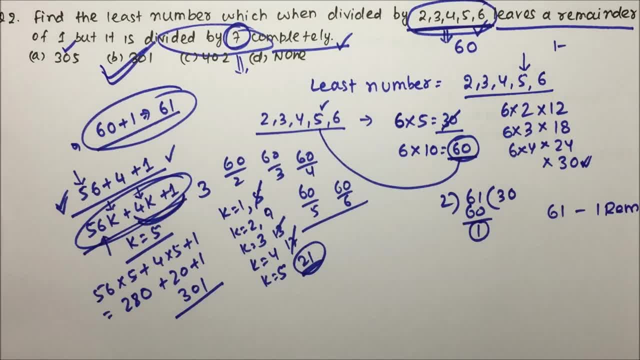 So 301 will be the number which will be divisible by, which will be divisible by 7.. Right, Okay, So 301 is the number. when we will divide by 2,, 3,, 4,, 5,, 6, it will leave a remainder. 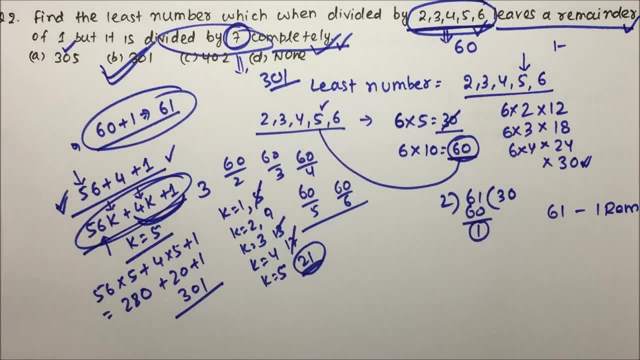 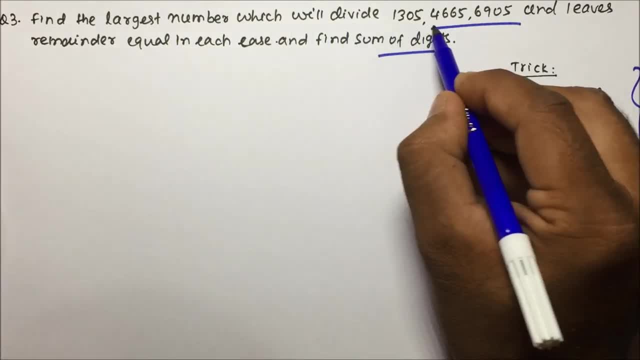 of 1 and it will be divisible by the. it will be divisible by the 7.. Right, It will be divided completely, Right? Okay, Now let's move to the question number 3.. Question number 3.. Find the largest number which will divide 1305,, 4665, 6905 and leaves remainder equal. 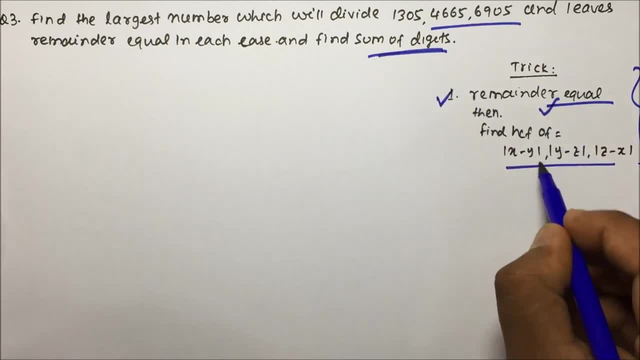 in each case and find sum of digits. So if remainder is equal, then your answer will be: then your answer will be: that means your largest number will be see largest number means hcf. Then the largest number, hcf, will be. so you have to calculate the hcf of x minus y mod. 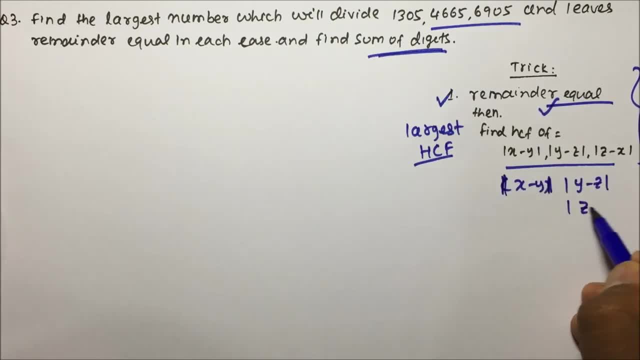 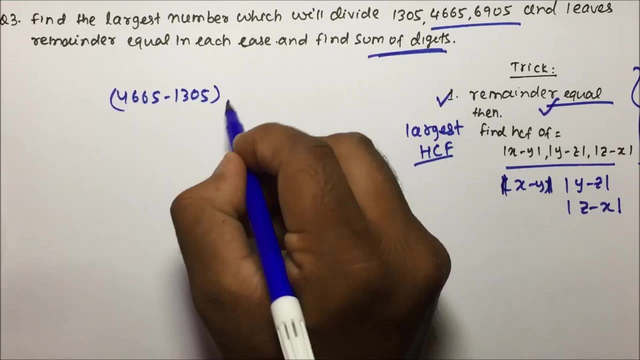 is there? Means you have to take the positive value, then y minus z and then z minus x, Right, Okay, So you can see. I will subtract 4665 minus 1305 comma. then I can subtract 6905 minus. 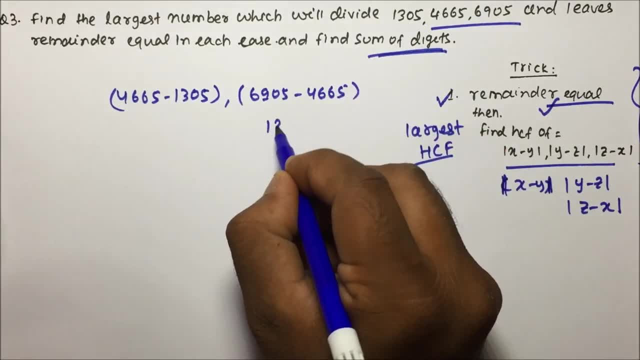 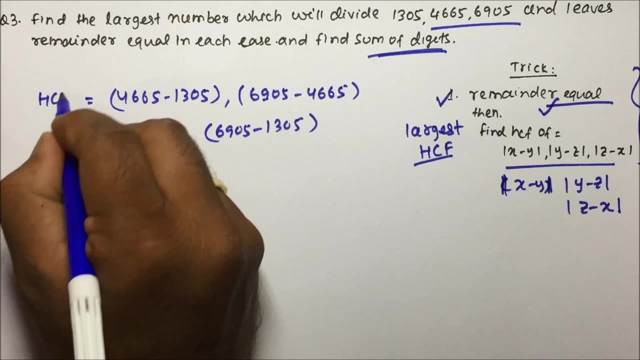 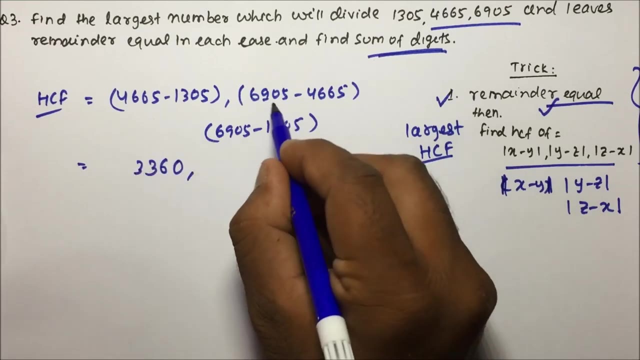 4665, then I can subtract 1305 from 6905.. Right, Okay, So this hcf, we have to calculate hcf. of this numbers, you have to calculate: 5 minus 5 is 0,, 6 is 6,, 3 and this will be 3.. 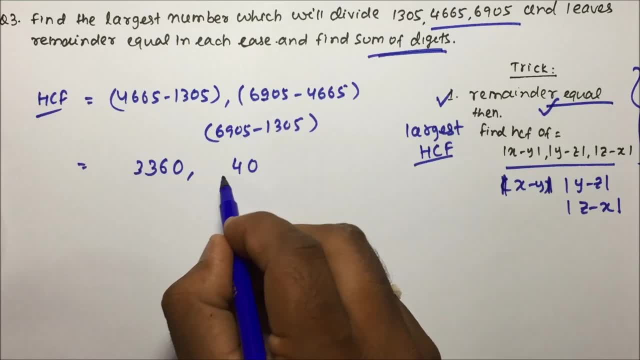 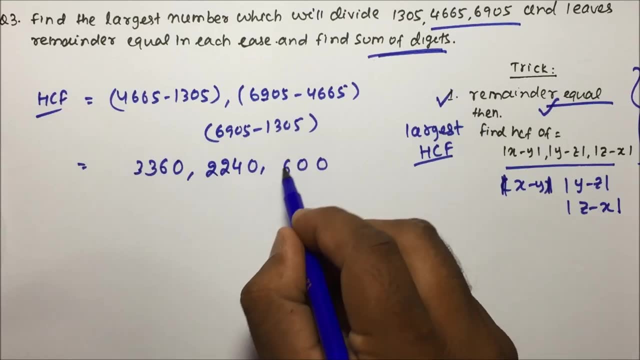 Then 5 minus 5 is 0.. 10 minus 6 is 4.. Then 8 minus 6 is 2 and 6 minus 4 is 2.. And then 5 minus 5 is 0,, 0,, 9 minus 3 is 6 and 6 minus 1 is 5.. 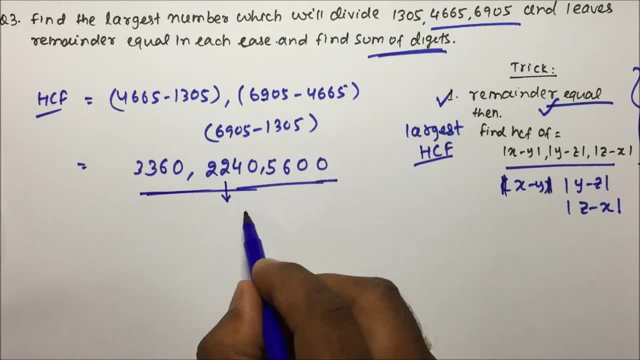 So what is the? you can see what is the smallest factor here. So a smallest factor is 2240. But 5600 will not be divisible by 2240. So what we will do, we will take the, we will take the another factor of this, so just. 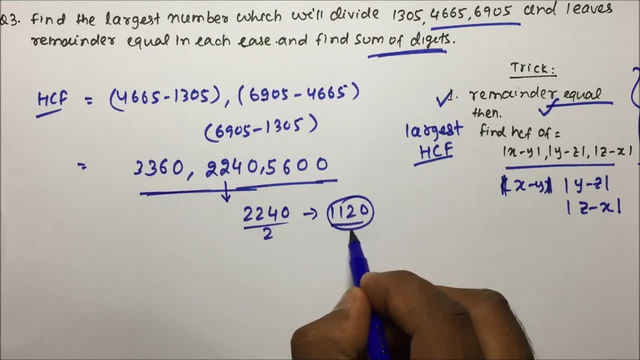 divide by 2, so it will be 1120.. Now you try to divide this numbers by 1120.. So if you will try to divide 3 times, 3 times this will get divided, then 2 times this will.